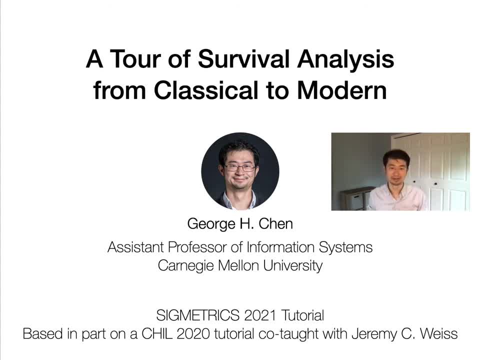 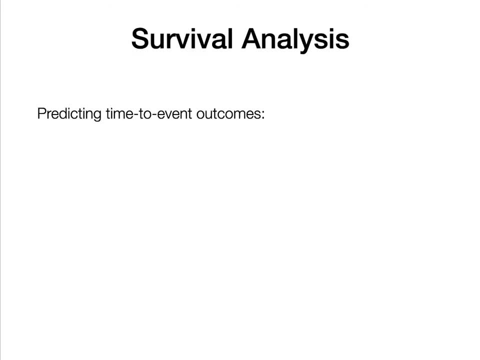 and the older version of this tutorial had much more of a health care focus. So survival analysis is about predicting time-to-event outcomes. Examples of these outcomes include time until death. time until a disease relapses. time until hospital discharge. Another way to put this would be hospital length of stay. 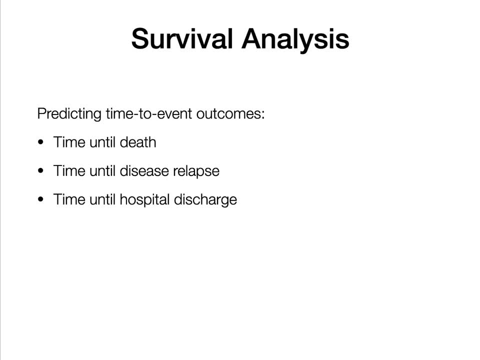 Time-to-event outcomes don't have to be about healthcare. To give two examples of time-to-event outcomes that are not healthcare-related, One would be predicting time until a convicted criminal reoffends. This is called recidivism. There's also predicting time until a user unsubscribes from a service. 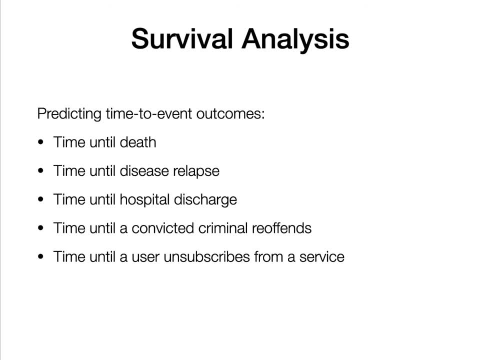 such as a movie or TV show streaming service or a music streaming service. There are, of course, many more examples of time-to-event outcomes In this tutorial. to keep the terminology easier to understand, I'm mostly going to phrase terminology in terms of this first example of predicting time until death. 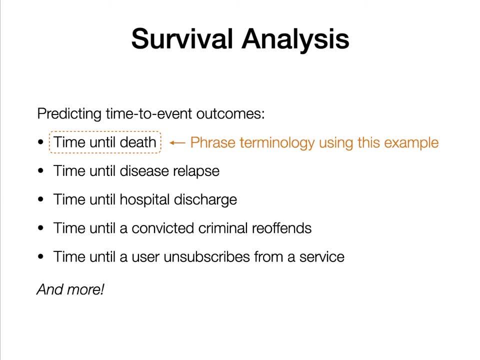 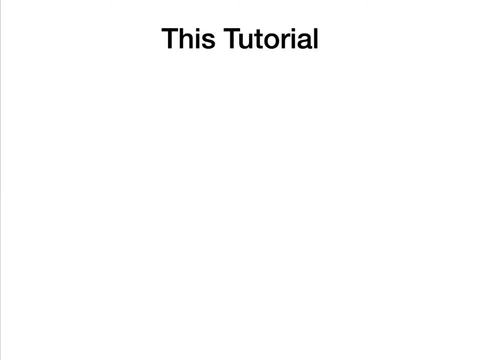 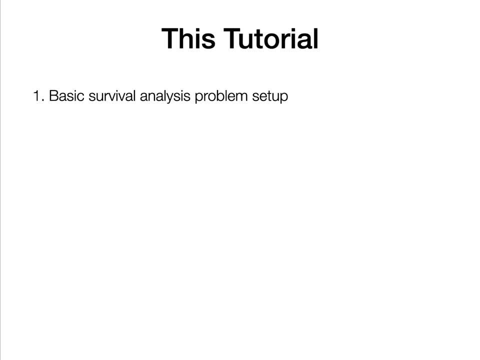 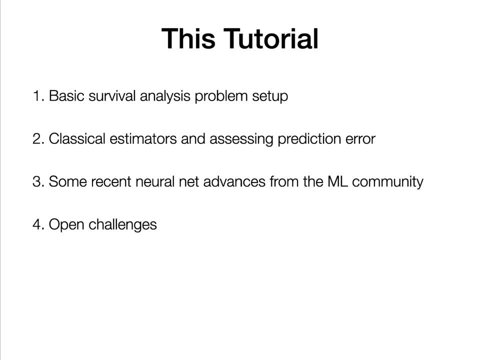 Finally, I will talk about open challenges At the end of this tutorial. I will point out some software packages And lastly, before getting started, I'll mention that all the material you're seeing here are posted on this web page. that's shown on the slide. 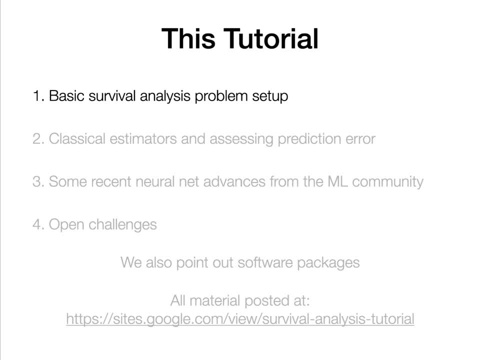 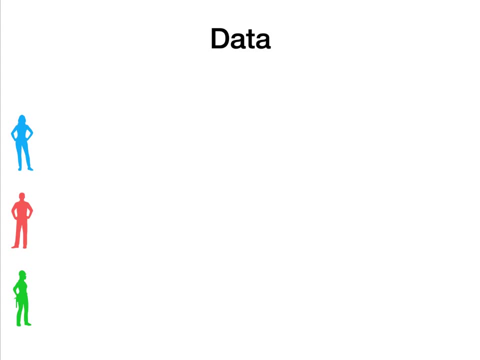 Alright, so let's get started with the basic survival analysis problem setup. In survival analysis, our data looks something like this: We have a bunch of patients or data points and we have a bunch of features. So this example that I'm showing you is a healthcare example And for simplicity here let's say: 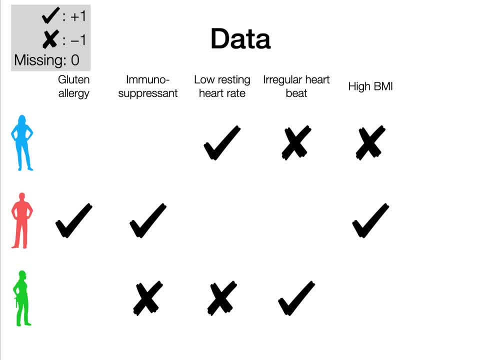 I have a measurement that are either a checkmark for a plus one, an x for a minus one, and if it's missing I put a zero. Of course you can have measurements that are not just binary or zero for missing. You can have continuous valued features And the label that we're trying to predict is the. 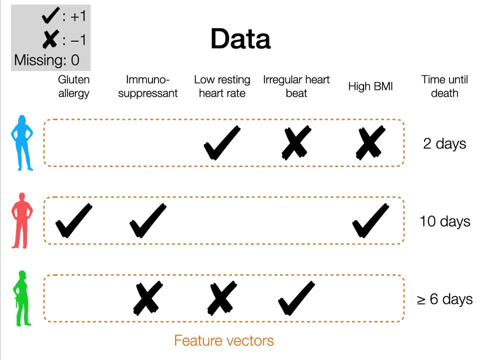 time and total depth. Okay, so basically we have our feature vectors and then we have these durations that we're trying to predict And note that in our training data, as is common in survival analysis, we typically cannot wait for everyone in the training data to. 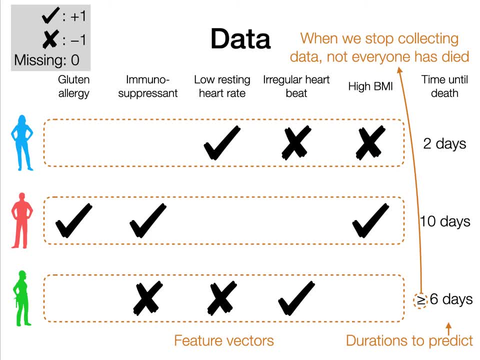 die. So that's why, for this last patient here, there's this greater than or equal to sign right here. This means that when we stopped collecting training data, this green patient was still alive, and that's why their time until death is at least six days. 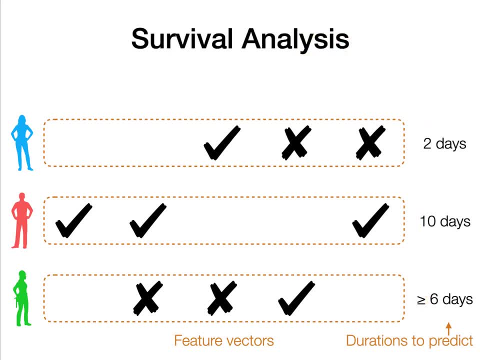 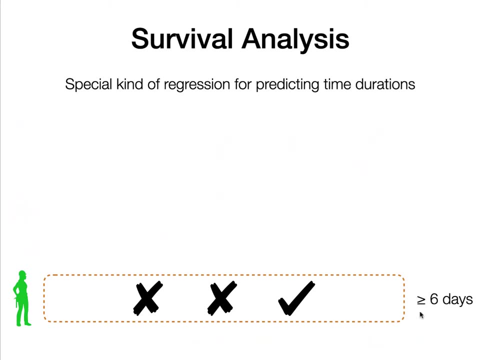 Okay, with that said, you can think of survival analysis as essentially like this: You can think of survival analysis as essentially like this: a special kind of regression for predicting time durations. These durations are always non-negative, and then we have this peculiar feature where we can have this greater than. 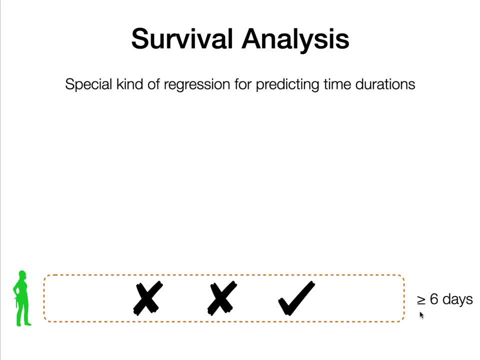 or equal to sign. Just to anchor some notation for the ith person, I will use xi to denote the ith person's feature vector. The next thing is, I will use yi to denote the observed duration. I'll also refer to this as the observed time. 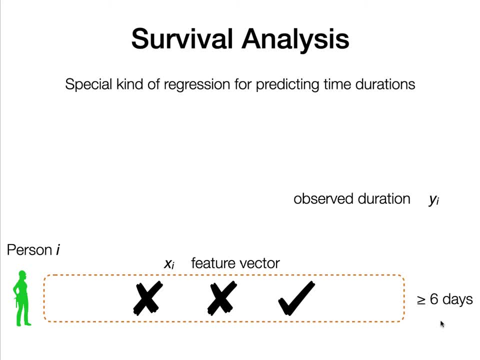 So yi for this green patient is equal to six. And then we also keep track of what's called the event indicator, delta i, which is, in this example, saying does the person die or not? in the training data, Because we have this greater than or equal. 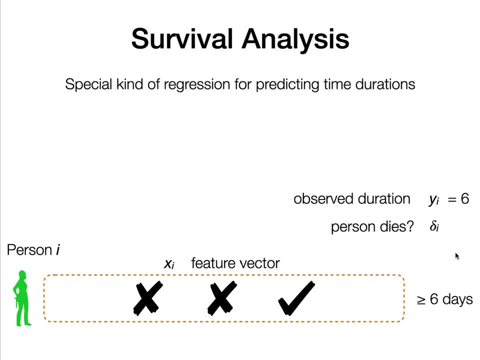 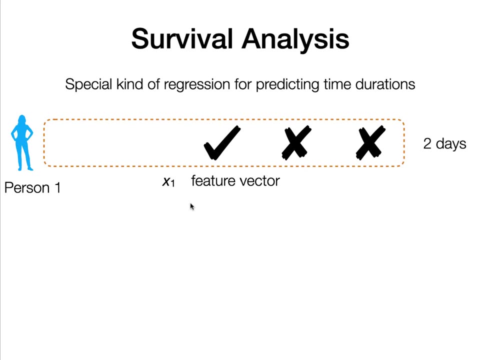 to sign. this patient was still alive when we stopped collecting training data, so delta i would be set to be equal to zero, meaning that death did not happen, Whereas for the first patient that we saw, person one, the feature vector would be denoted as x1,. 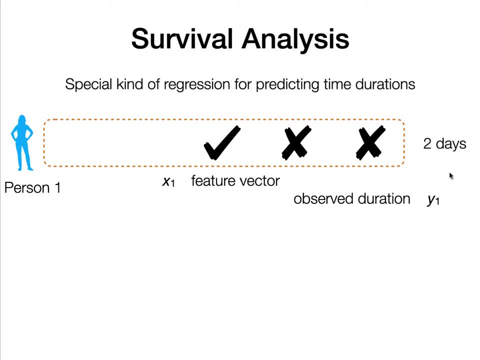 and the observed duration y1 is, in this case is, equal to two, And, whether the person dies, the event indicator, delta i, is equal to one. in this case, We don't have the greater than or equal to sign. We actually do observe the time until death. So, with that being said, we have our training data. 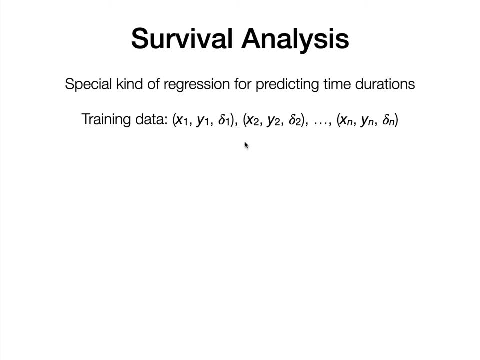 which consists of the feature vectors, the xi's, the observed durations or observed times, the yi's and the event indicators, the delta i's. And what we want is for a new patient or a new data point with feature vector x. okay, so a test feature vector x. we want to be able to predict the. 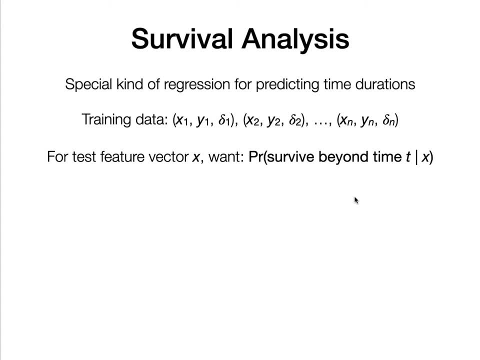 probability of surviving beyond time. t condition on the feature vector x. Okay, so this I'll be referring to throughout this tutorial as s given x, also called the survival function or survival curve. Note that this is a function of time, and so a survival curve looks something like this: 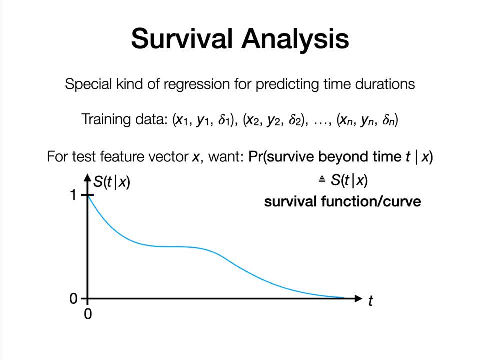 Okay, note that, unlike in the standard regression setup, we're not just predicting a single time, we're predicting this whole curve. And this curve: note that it monotonically decreases. It starts at 1, And then it decays to zero. 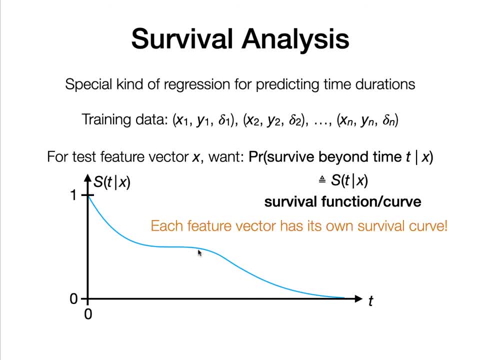 OK, the other thing I'll say is that we have different survival curve for each feature, vector X, And also, if you did want a point estimate for the survival time. there are different ways to back it out. Once you know us, I'll give you two example ways of doing this. 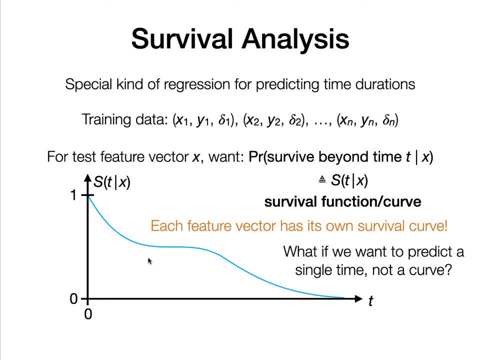 One way is you look at where this curve, this blue curve, crosses one half- OK, where it crosses one half, and you look at the time. this is referred to as a median survival time estimate for feature vector X. OK, as another example of how you can back out a point estimate for the survival time is you can look at the area under this blue curve. 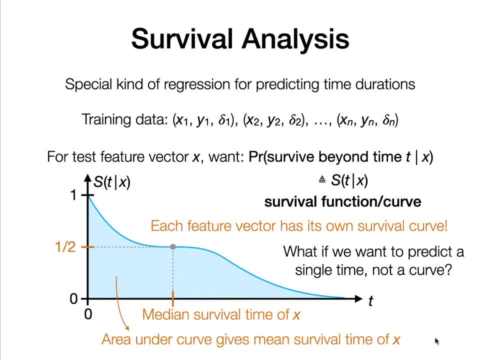 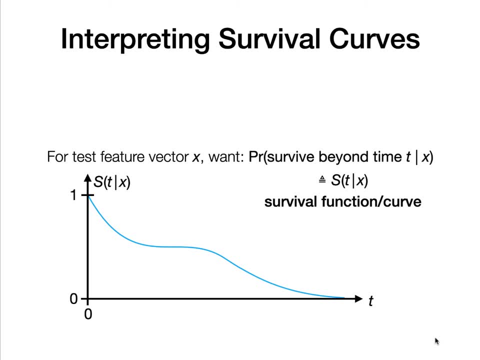 OK, and this gives an estimate of the mean survival time for a feature vector X. So I'll say a little bit About interpreting these survival curves. what the time to event outcome is matters here, OK. so for example, if the outcome is time until death, then typically longer is considered better. 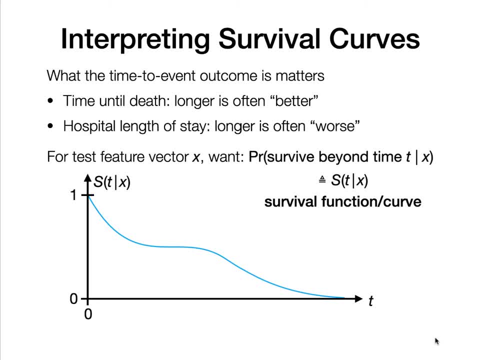 OK, whereas if you are looking at an outcome such as hospital length of stay, usually longer is considered worse. So, depending on your time to event outcome, you need to have some idea of direct Now whether longer time until your event is considered better or if it's considered worse. 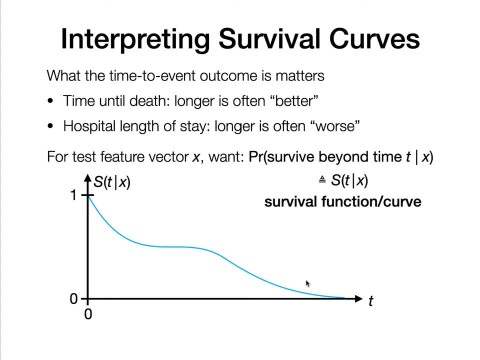 So, with that being said, we have this blue curve here for a different feature vector. Perhaps the survival curve looks like this purple curve here. OK, and so if the outcome is time until death, then we would typically say that the purple curve is uniformly worse than blue, because the probability of surviving beyond any time T is less than 1.. 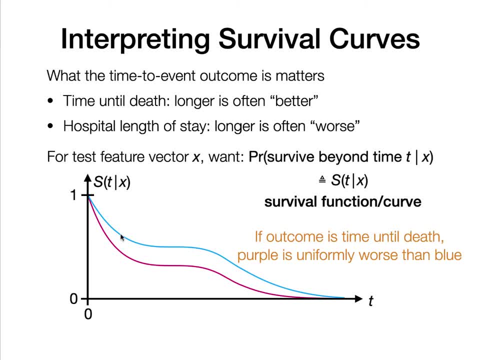 OK, And so if the outcome is time until death, then we would typically say that the blue curve is less than the corresponding value for the blue curve. OK, of course, it's not always a case that you have one data point- survival curve- being uniformly better or uniformly worse than another. 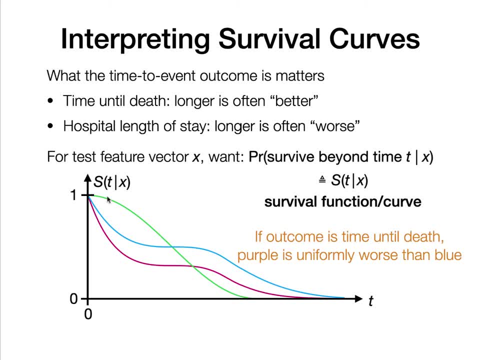 You can also have this behavior where, for a different feature vector, the survival curve can be this green curve, where it's not always better than or worse than the blue or purple curves. OK, so sometimes it's better, Sometimes it's worse. And of course you can also, instead of comparing the different curves, you can compare the mean survival times to the areas under the three different curves here, or you can compare the medium survival times. 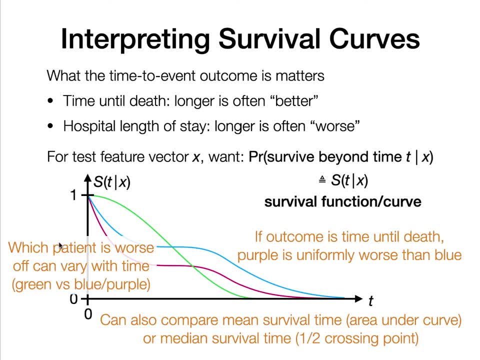 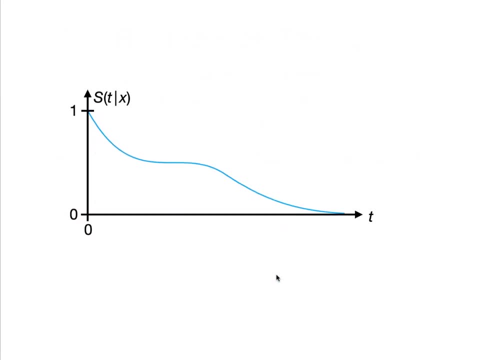 So you look at the times at which each of these curves crosses one half and you compare them to see which curve has smaller median survival time versus larger median survival time. OK, All right. So the next thing I'll say a little bit about is theory. 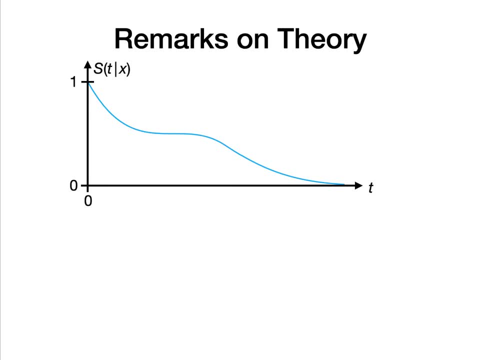 In this tutorial. I'm not going to go into any sort of details on theoretical guarantees, but it's good to know a little bit about when we should even expect the estimators to work well. So one thing that is the case is that we cannot estimate the survival curve arbitrarily accurately for all of time. 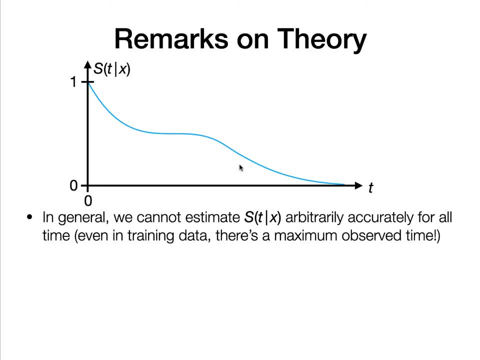 OK, OK. One intuitive way to think about this is that even in the training data there's some maximum Observed duration that we see. So for values of T larger than that maximum observed duration, our estimate for the survival curve will just be some sort of extrapolation. 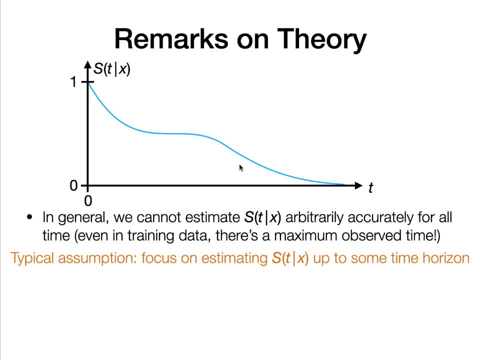 OK. So typically in theoretical analyses people will focus on estimating S of T, given X, accurately, just up to some time horizon. So another thing I'll say is that the censoring mechanism and also the censoring rate do matter a lot. OK. 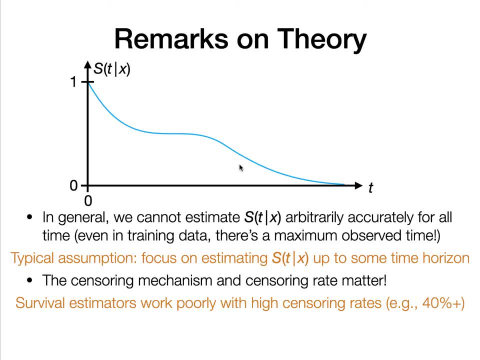 OK, OK. So just to give an example: basically, survival estimators will tend to work poorly if you have high censoring rates. What do I mean by this? For example, if you're predicting time until a hard drive fails or time until a musician gets signed by a record label, both of these prediction tasks are very hard. 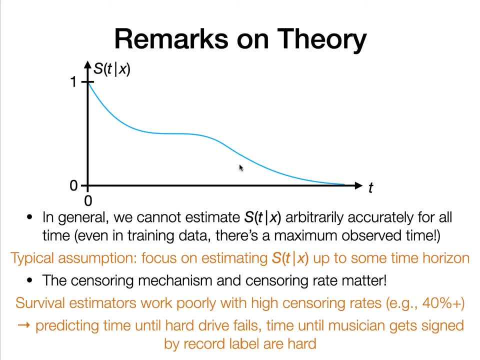 And part of the difficulty is that very, very few hard drives fail Right, So the percentage of data points you have that are not censored, for which you actually do see The time until failure, is going to be very, very, very tiny. 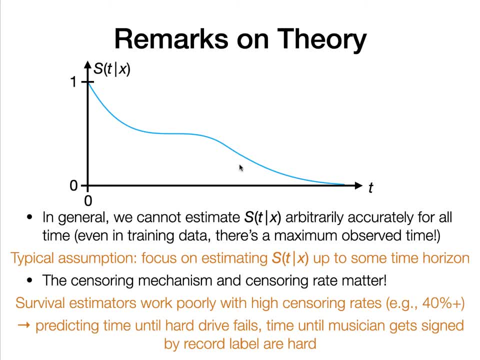 Similarly, among artists trying to get signed by record labels, the fraction of them that actually do get signed is extremely small, And so if you're trying to predict time until the musician gets signed- most musicians- they're going to be censored at any point. 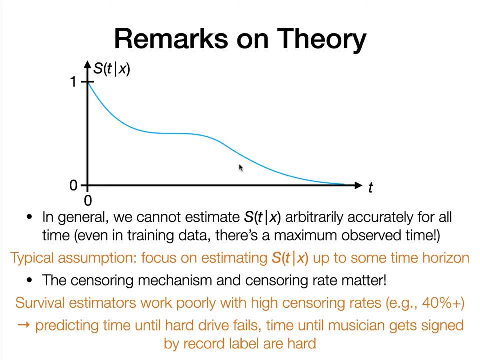 If you stop collecting data. most musicians didn't get signed yet. OK, So if you're in those regimes where you have high censoring rates, you're going to run into trouble, And if you don't, you're going to be censored. 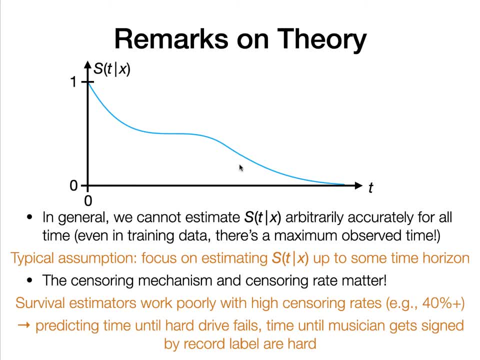 And if you do want to do prediction in those settings, I would recommend first solving a simpler classification task to basically narrow down the cohort of people or hard drives that you're looking at to the ones that have a higher fraction of failure, And then among those, you do some sort of time to event prediction. 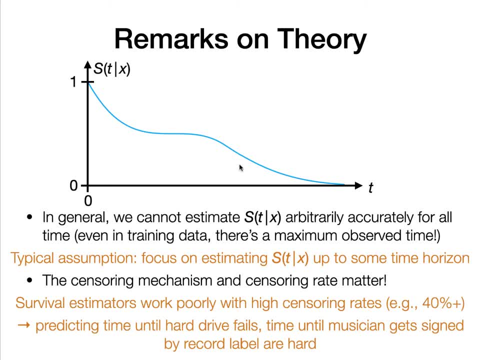 OK because, like I said otherwise, survival estimators- these typically don't work well if you have high censoring rates. By the way, what I put on the slide here Is it's kind of a made up number of what's considered a high censoring rate. kind of varies by application and method and so forth. 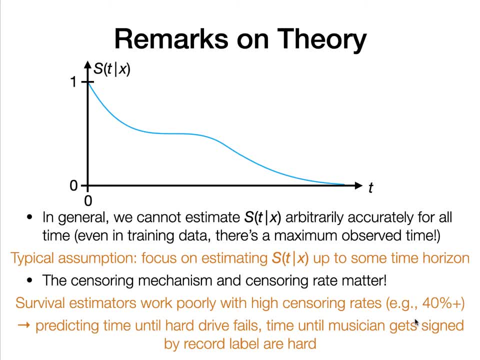 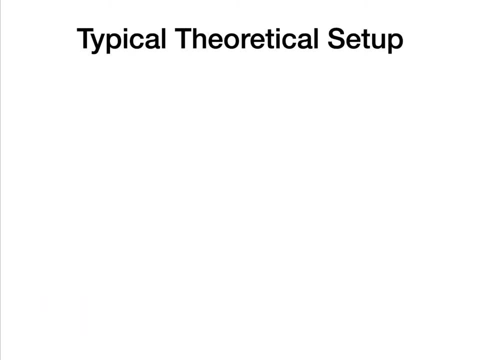 In a lot of papers, 40 percent or higher would be considered like a fairly high censoring rate already. Something else I'll briefly say is what the typical theoretical setup is. So, just like with standard regression and classification theoretical analyses, we assume that the data are generated IID. 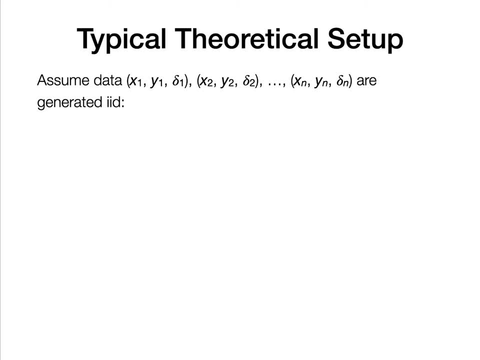 But now it's a little bit More complicated because we have censoring. So the typical assumption is that each of the XIs are sampled from some feature distribution. This part, it would be the same as in classification and regression. However, the next thing that becomes different is we assume that we sample a true survival time ZI in a true censoring time CI. 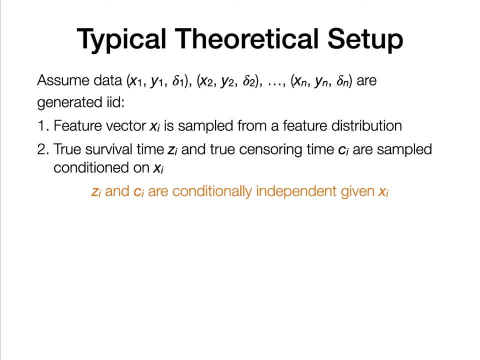 And these are sampled in a white condition on XI. OK, And importantly, a key assumption is that the true survival time in the true Time are conditionally independent given XI, and then if the survival time is less than the censoring time mean that death happens before censoring. then we set the observed YI value to be equal to the survival time ZI and we set the event indicator to be equal to one. 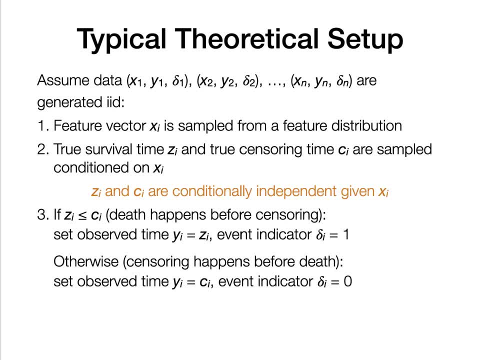 OK, otherwise. so censoring happens before death. then we set the observed time YI to be equal to CI and the event indicator to be equal to one. OK, So we set the observed time ZI to be equal to zero. OK, so this just gives you an idea of the typical theoretical setup. 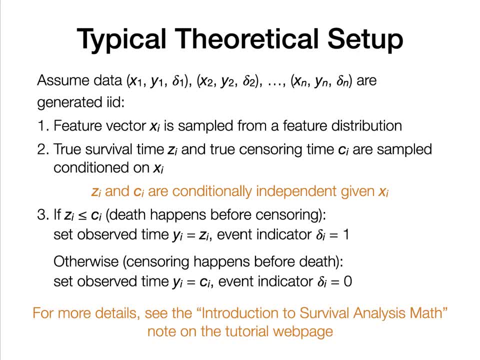 This is referred to as random censoring. OK, I'll say for more details on not just this but also other basic survival analysis math concepts that I mentioned in the tutorial. they are posted in a note on the tutorial web page. The note is titled Introduction to Survival Analysis Math. 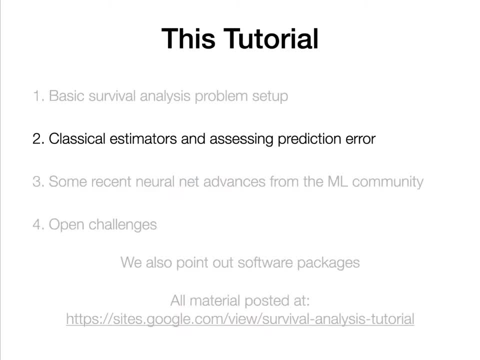 OK, All right. so, with that being said, now we'll move on to the second part of the tutorial, where we're going to talk about how to actually estimate the survival function and also how to assess prediction error. Okay, so here's an example of a survival estimator. 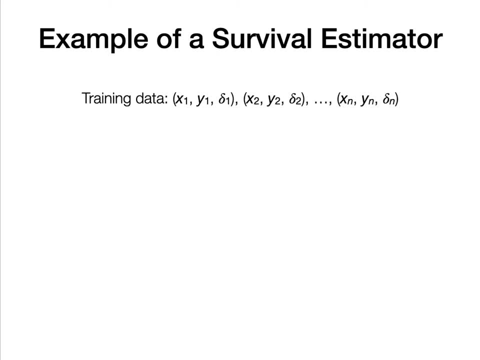 We're going to do something that looks kind of dumb, but we'll get to the more realistic setup momentarily. We'll begin by ignoring all the feature vectors. okay, Then of course, the survival function that we estimate is not going to be conditioned. 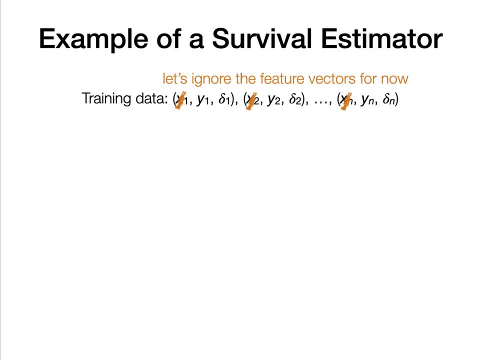 on the feature vector. So that's okay. We'll see what happens in a moment. What we can do is we can look at all the unique observed times in which there was actually a death that occurred. okay, So I'm going to call those T1, T2, all the way up to T, capital L. 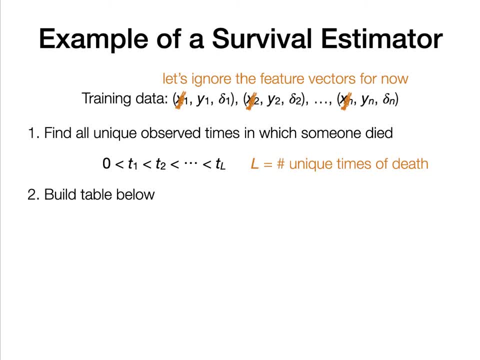 We're in T1,, T2, all the way up to T, capital L- The number of unique times of death- Then what I'm going to do is I'm going to build the following table, So I have my different times: T1,, T2, up to TL- and at each of these time points I'm 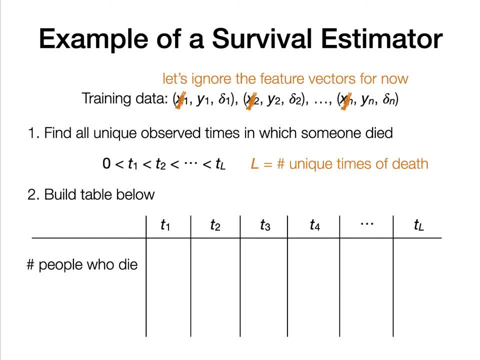 going to keep track of how many people died at that time point. okay, So this will be D1, D2, D3, all the way up to DL. The other thing I am going to keep track of is the number of people that were killed. 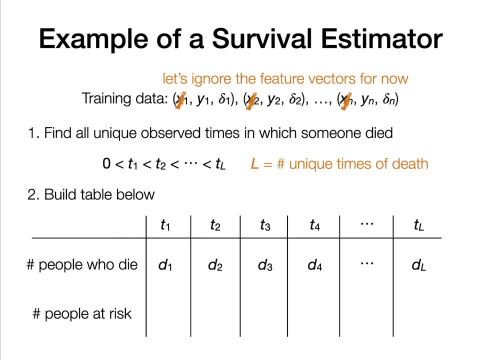 This is the number of people that are at risk. okay, This is the number of people that could possibly die at these different time points, and I'll call these N1,, N2, N3, all the way to NL. okay. 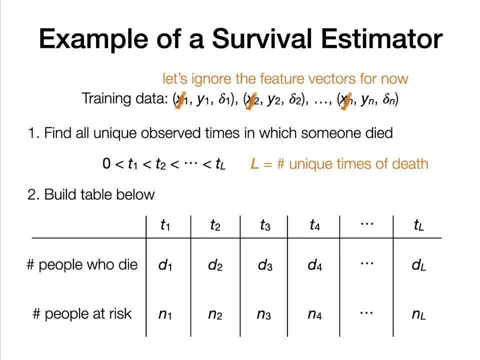 So I'll just say this part neatly handles centering in the following manner: So N2 is not necessarily equal to just N1 minus D1, okay, N1 is typically going to be equal to the total number of training examples N. but you know. 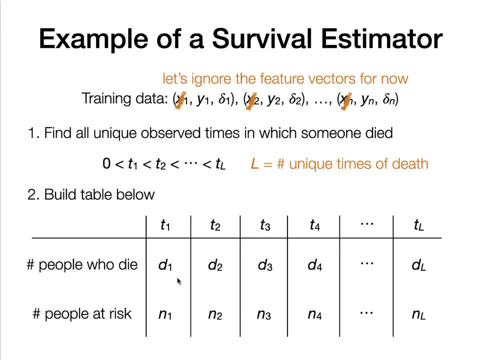 some people die, but also some people can get censored. They drop out of the study and after you subtract D1 from N1 and also subtract the people who dropped out of the study, that gives you N2, okay, So in that sense this table actually neatly accounts for censoring. 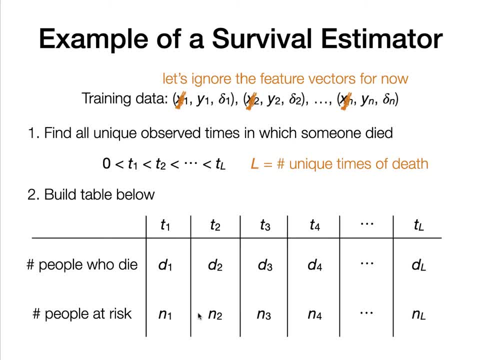 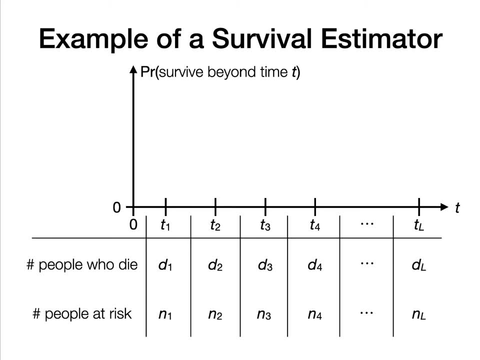 Okay. So, with that being said, Now what we can do is: well, we have this timeline and we're going to estimate the probability of surviving beyond time T. Again, this is not conditioned on a feature vector, because we're ignoring feature vectors for now. 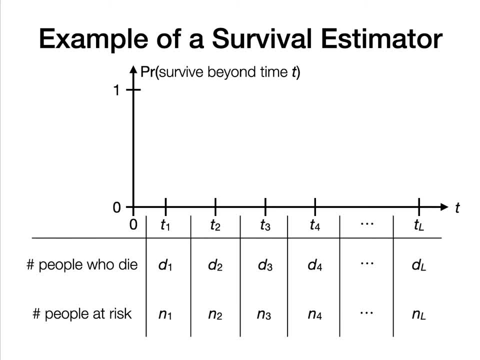 And so initially, well, initially, we don't see anything from time 0 to time T1, so we'll just guess that the probability of surviving beyond these particular times, we'll just estimate it to be 1,. okay, And then the probability. 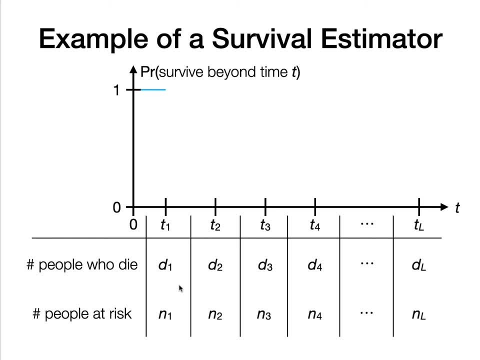 Oh, The probability of dying at time T1 is well, it's D1 divided by N1. And so the probability of not dying at time T1 is 1 minus D1 divided by N1,. okay, And so the probability of surviving beyond time T1 is going to be this: 1 minus D1 divided. 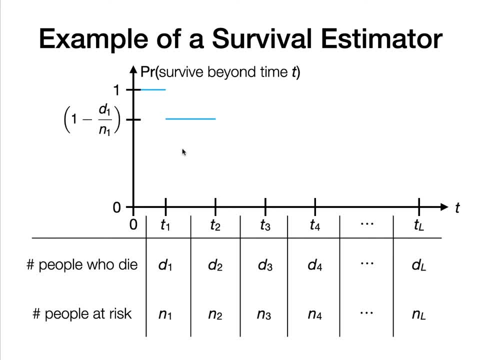 by N1.. And, using this same logic, when we get to time T2, the probability of surviving that is going to be, Well, it's going to be the probability of surviving from time T1 to time T2.. So the probability of surviving from time 0 to T1, which is this: first, 1 minus D1 over. 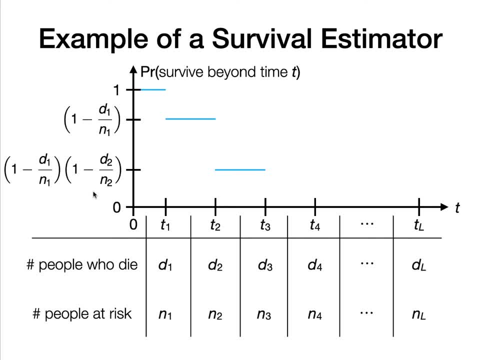 N1 term times the probability of surviving from T1 to T2, 1 minus D2 over N2, and so forth. In general, the equation looks like this: We're multiplying the empirical probabilities of surviving from time 0 to T1,, T1 to T2,. 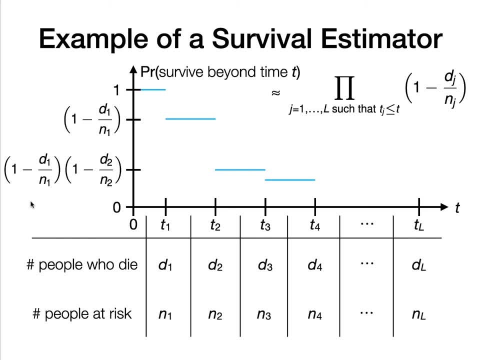 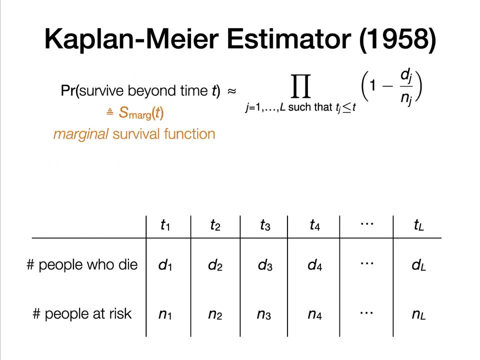 T2 to T3, and so forth, all the way until time little t that we plug in here. Okay, This thing has a name. This is the classical Kaplan-Meier estimator. I'll refer to this as estimating the marginal survival function, because it doesn't depend. 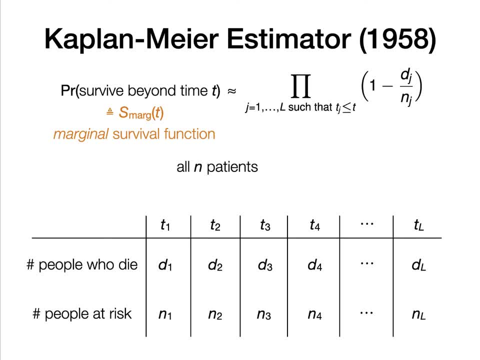 on feature vectors. You can think of this: as you have all N of your patients, you ignore their feature vectors and then you just throw them into this Kaplan-Meier estimator and you get this estimate of the survival curve out And there's a very, very simple way to account for feature vectors. 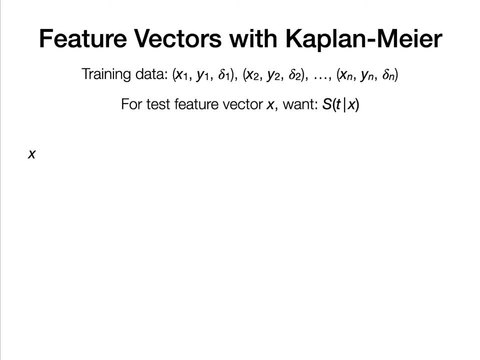 So what we're going to do is for a test feature vector x. we're first going to find the k training feature vectors that are closest to x. Okay, So that will give us k training patients. And if you then plug in their yi and delta i values into the Kaplan-Meier estimator, 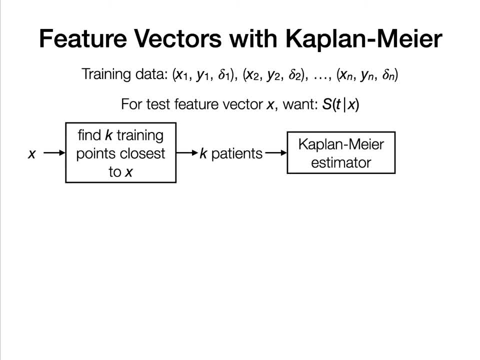 okay. So, again to be clear, we're applying the Kaplan-Meier estimator restricted to k, different patients' data points. Okay, So this is an estimate of a survival curve and this estimate does depend on this input test feature. vector x: 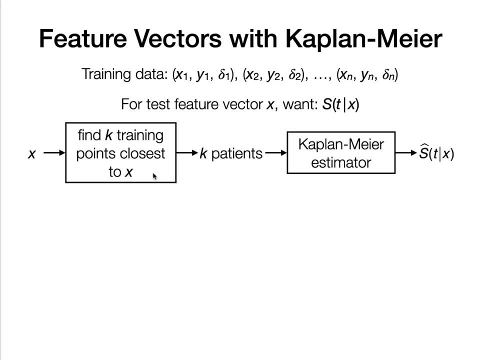 Okay, Because we're doing this nearest neighbor search thing here. Okay, Of course this generalizes to weighted k nearest neighbor variance. and also there's a kernel version of this kernel Kaplan-Meier estimator. In general these are referred to as conditional Kaplan-Meier estimators and these are by. 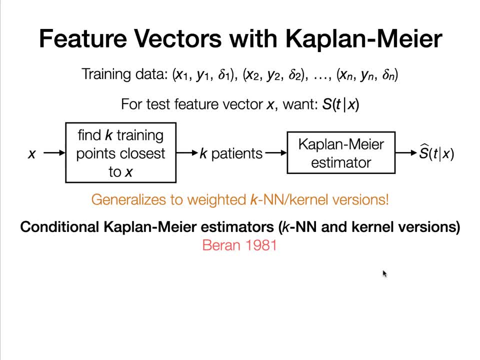 Bayron from back in 1981.. Okay, And I'll just say that, how well these k nearest neighbor and kernel conditional Kaplan-Meier estimators, how well these estimate the true survival curve S of t given x is well understood. I'll just say I have a paper from 2019 that gives finite sample error bounds, but even 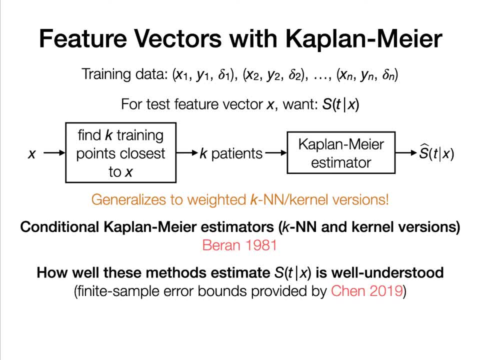 before I came up with this from decades ago, people have come up with asymptotic error bounds. Okay, Okay, Okay. So these are the two ways that we can use the non-parametric methods, meaning that we are not assuming any sort of parametric form for the survival curves. 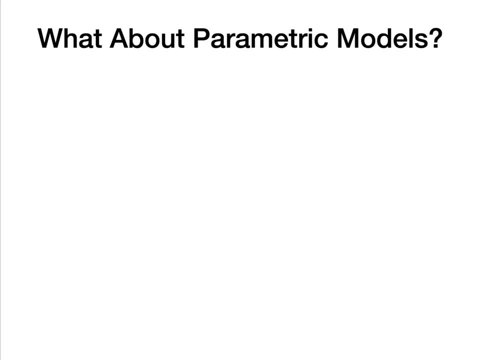 So you might then wonder: well, what about parametric models? Before I get into the only partly parametric model that I'll talk about in this tutorial, I'll mention that there are some common variants of the survival curve that are commonly used. 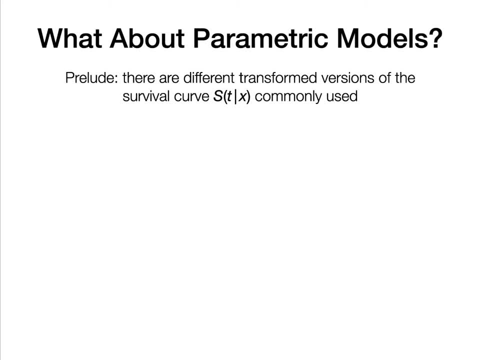 and commonly estimated. Okay, In a sense, that'll be made clear momentarily. these different transform versions are kind of equivalent. Okay, So we have our survival function, S of t given x- I can take the negative log of this- and this thing is referred to as the cumulative hazard. 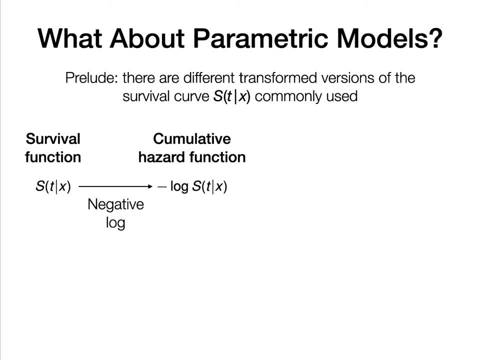 function, And I'll say in a little bit why it's called that. but for now I'll just say this is a cumulative hazard function. Then I can take the derivative with respect to time, Okay, And when I do that I'm going to get something called the hazard function. 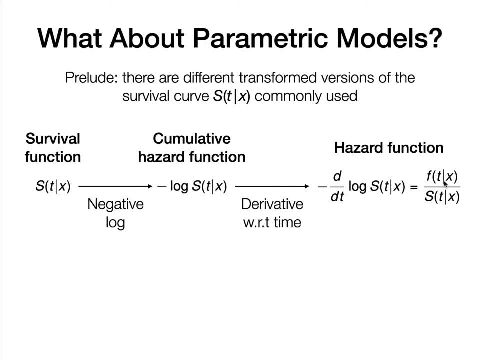 The hazard function turns out to be equal to. in the numerator I have this little f of t given x. This is the probability density function of the survival time, being little t given the feature vector x. Okay, And you can easily interpret what's happening in this right-hand side equation. 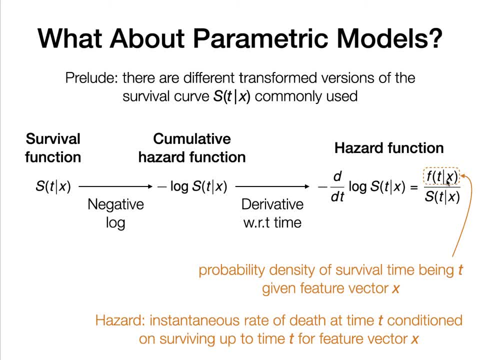 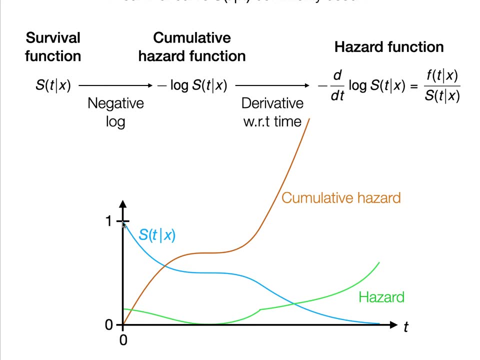 It's the instantaneous rate of death at time t. Condition of death. Condition on surviving up to time t. Okay, All for feature vector x. All right, So just to give you an example of what these different functions look like when the blue 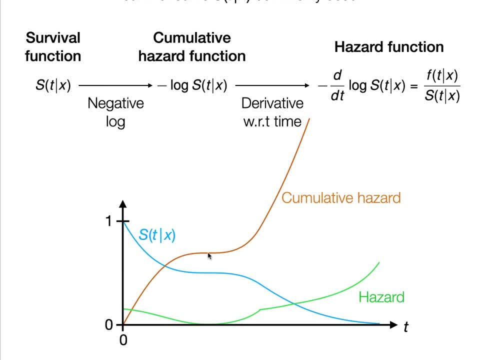 curve. here is the survival function which, again, it monotonically decreases from one to zero. For the blue curve, the corresponding cumulative hazard function is this dark orange curve, Okay, Which is also a monotonic function, But instead of monotonically decreasing, it's monotonically increasing. 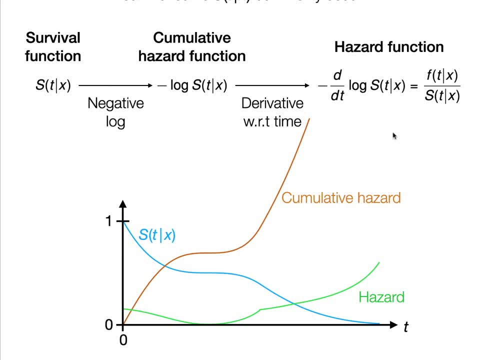 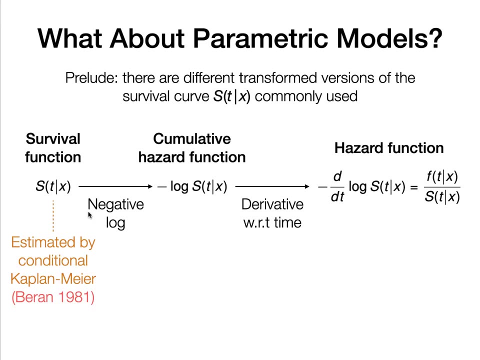 Okay, And then the hazard function is well, the hazard function doesn't actually have to be a monotonic function And, as you can see here, it decreases and then it increases. So, in any case, these are examples, And we just saw that the conditional Kappen-Meier estimator can estimate the survival function. 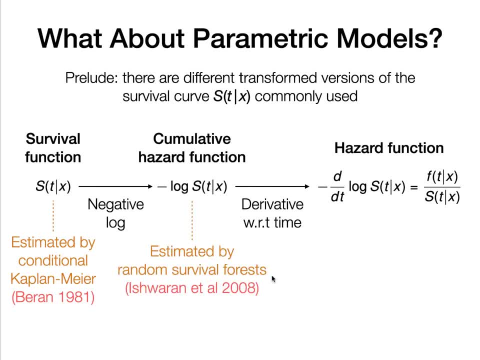 The cumulative hazard function can be estimated, For example, By random survival force. These are the random force analog for survival analysis. Okay, And back in the original random survival force paper. they focus on estimating this cumulative hazard function. Lastly, we also have this hazard function and this is estimated by the model that I'll 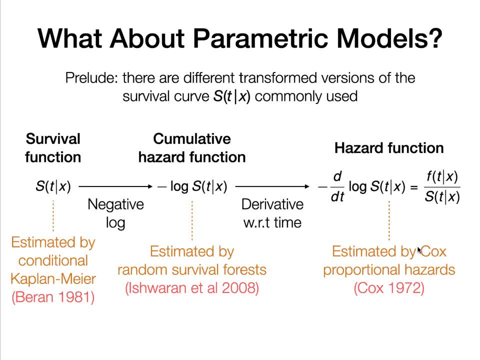 spend a bit of time talking about next, which is called the Cox proportional hazards model. Okay, The left two things. These are examples of nonparametric methods. Again, These do not assume a parametric form for the survival function S In the Cox model, as we'll see shortly, it's partly parametric in a sense that I'll make 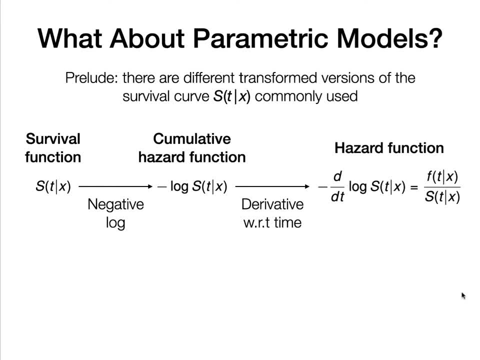 clear in a moment. So before moving on I'll just make this part clear. We can go from the survival function to the cumulative hazard function, to the hazard function. We can of course go backwards If I call the hazard function little h of T given X. 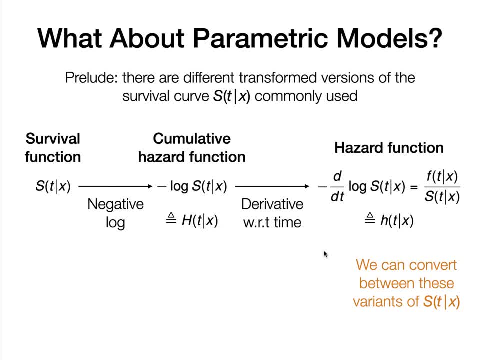 If I call the cumulative hazard function Kappen-Meier, If I call the cumulative hazard function capital H of T given X, then I can of course integrate with the respective time to go from the hazard function to the cumulative hazard function. Okay, 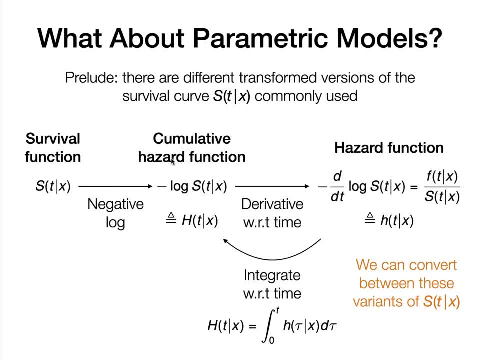 So now I mean, you can see, the cumulative hazard function is called the cumulative hazard function because we're summing the hazard function, We're doing this integration to go from this right thing to this middle thing. Okay, And then we can negate and exponentiate to convert the cumulative hazard function to 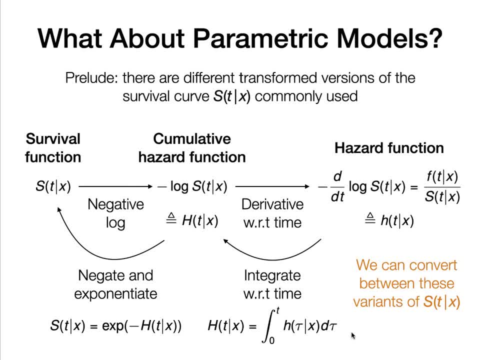 the survival function. Okay, So this is the sense of why these are in some way equivalent. If we have an estimate of any of these three things, we can come up with an estimate for the other two things. okay, Possibly requiring, you know, let's say, numerical integration or something like that. 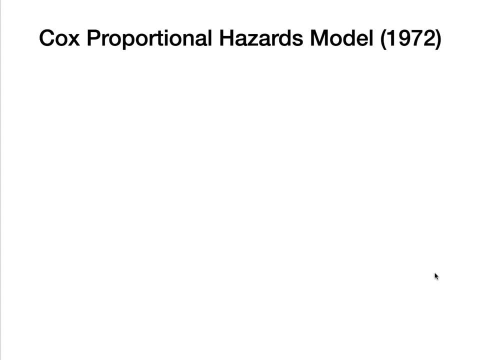 All right. So now I'm going to talk about the Cox proportional hazards model and the reason why I'm going to focus on this, Because it is extremely popular. This is essentially the linear regression of survival analysis, although, as you'll see, 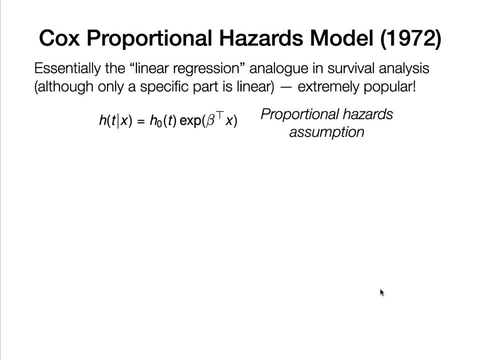 only part of it is linear. So the underlying assumption is called the proportional hazard assumption and it basically assumes that the hazard function is of this form. okay, It decomposes in this particular way and the parameters here are the non-negative function H sub zero. 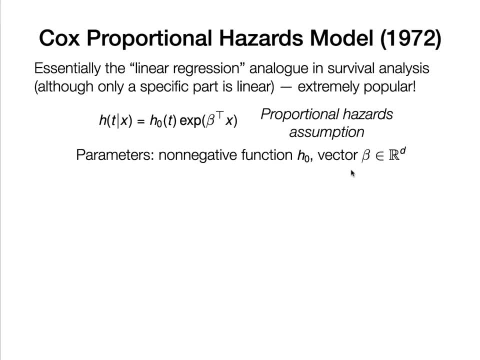 This is called the baseline hazard function and there's also an underlying parameter vector, beta, okay- Which is d-dimensional, where d is also the dimensionality of the feature vectors, okay, of these x's. It's called a proportional hazards model because, as you can see from the proportional hazards, 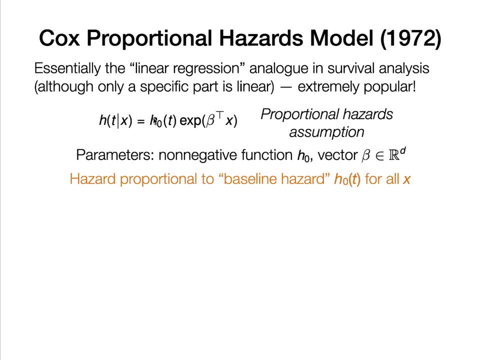 assumption: the hazard function is always proportional to the baseline hazard H sub zero for all values of x. Okay, This is referred to as a semi-parametric model because typically no parametric form is assumed for this H sub zero. okay. 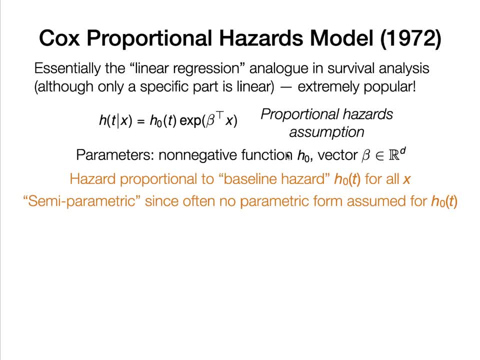 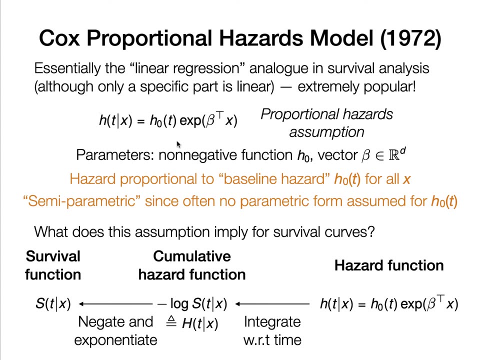 You could assume a parametric form, but it's just very common for people not to assume a parametric form for H sub zero. Okay, well, what does making this proportional hazards assumption mean in terms of the survival curves? Well, it means the following: recall that once we specify the hazard function, we can 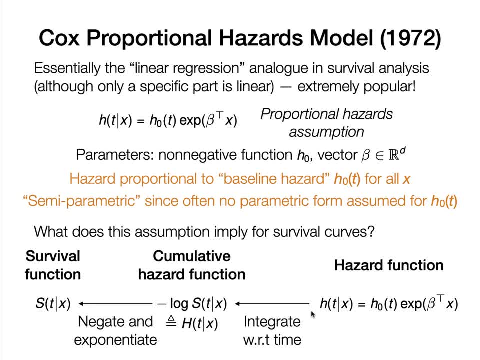 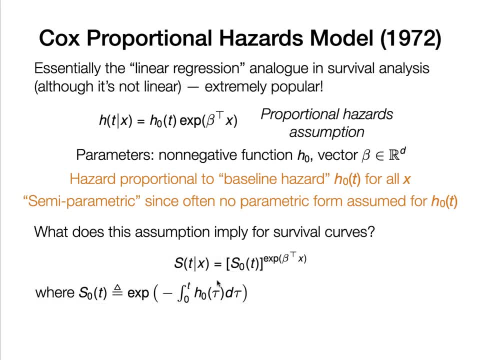 go backwards, We can back out the survival function, and if you do this thing right here, you integrate and then you negate and exponentiate, then what you'll find is that the survival curves that are possible under a proportional hazards assumption must necessarily be powers. of what? 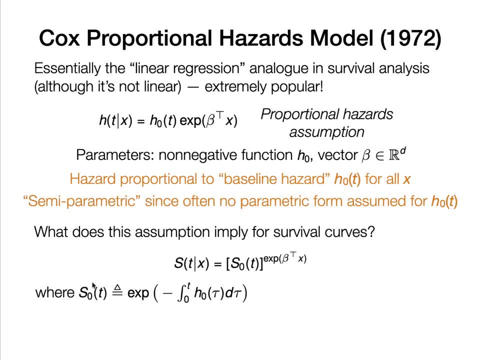 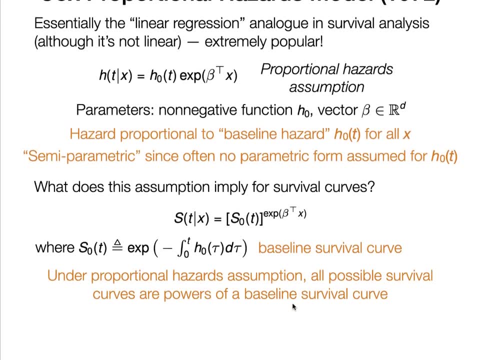 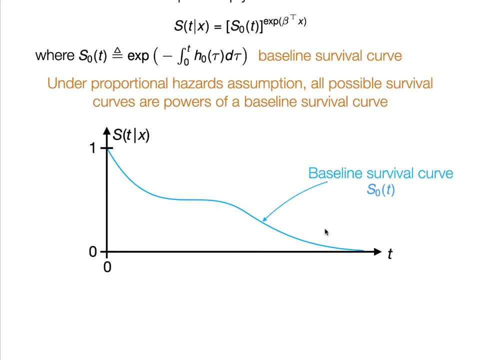 I am going to call a baseline survival curve capital S sub zero. Okay, Um, So Okay. What that means is, for example, if this blue curve is your baseline survival curve S sub zero, then under a proportional hazards assumption, all survival curves that are allowed have. 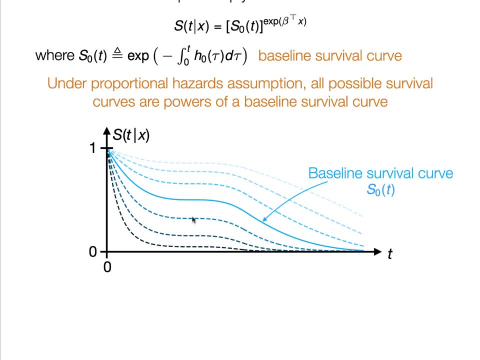 to be powers of this curve. So in particular, they have to look like these dotted lines: okay, Where, as you have bigger positive values, of beta, transpose x, you're going to have survival curves. If you have more than one, you're going to have a survival curve. then you're going to 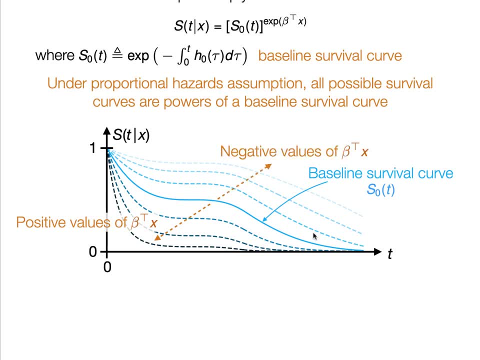 have a survival curve against one or more than one, which is closer to the origin, Whereas if you have very, very negative values of beta, transpose X, you're going to have survival curves that are getting closer to just being all one. Okay. 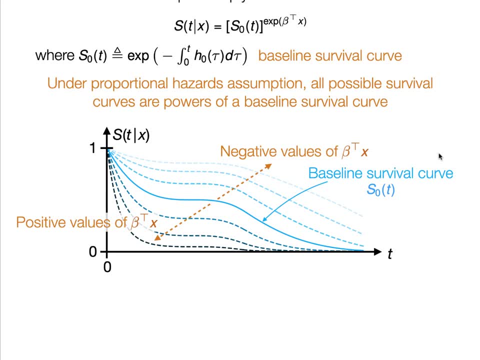 So here I'll just say: higher beta transpose X is then going to imply, in the case where the time to event outcome is, uh, let's say, time until death, then higher beta transpose x means output, means that we're moving closer to the origin and it means that we have a uniformly worse survival. 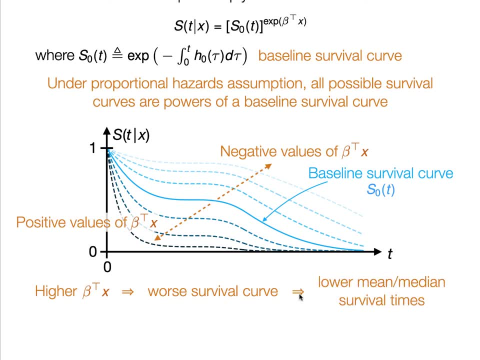 curve, OK, and that also means that if we look at the mean or median survival times, it's going to be shorter. OK, so that's what is happening here. The green curve would not be possible under a proportional hazards assumption if your baseline survival curve. 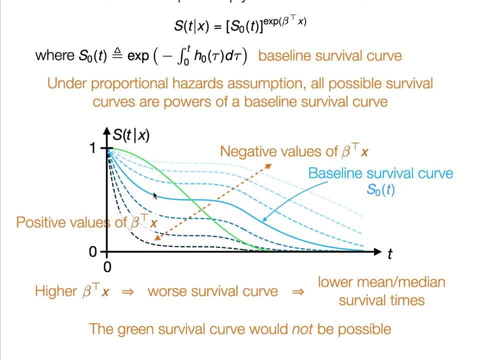 S sub zero. is this solid blue curve in the middle here? OK, so basically you cannot get crisscrossing behavior under the proportional hazards assumption, And I'll just say this is a key reason for why researchers might say that the proportional hazards assumption is restrictive. 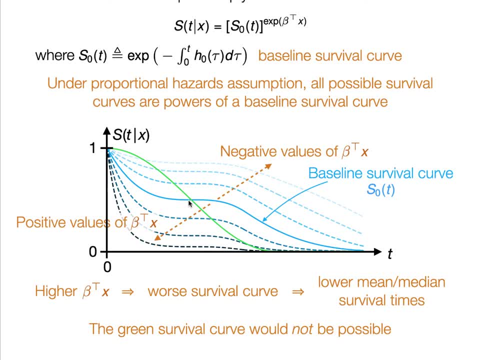 And it's because, well, oftentimes in real survival analysis data you can have for different feature vector survival curves that crisscross, like this green and blue curve. OK, so in that way we're going to be able to figure out what's going to happen, So we're going to be able to. 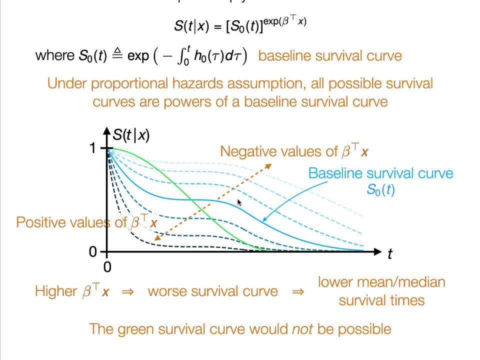 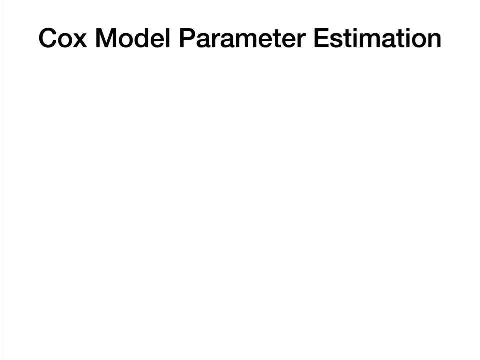 So in that way we're going to be able to figure out what's going to happen. So in that way case, the Cox model cannot actually handle this, And so you would have to turn to a different model. All right, now I'll say just a little bit about parameter estimation for the Cox model. 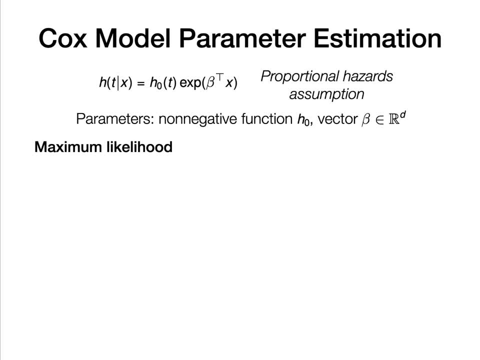 So how this works is basically its maximum likelihood OK, and it turns out that the standard way people do this will be to estimate beta without knowing H sub zero. the baseline hazard function OK, and it amounts to minimizing a convex loss. So here I'll just say you can use like Newton-Raphson is one of the standard ways people 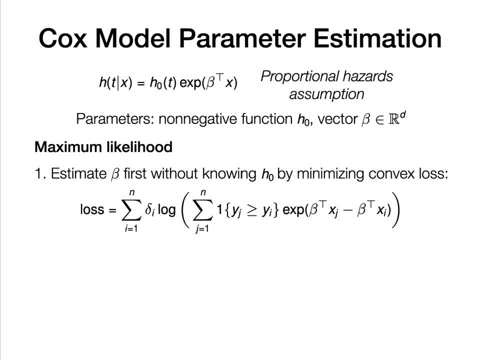 do it, But of course you can also use stochastic gradient descent. OK, and of course, if you wanted to, you can add, like a LASSO RAGE or elastic net regularization on beta, the regression coefficients. After you estimate beta, there's a standard procedure for estimating the baseline hazard. 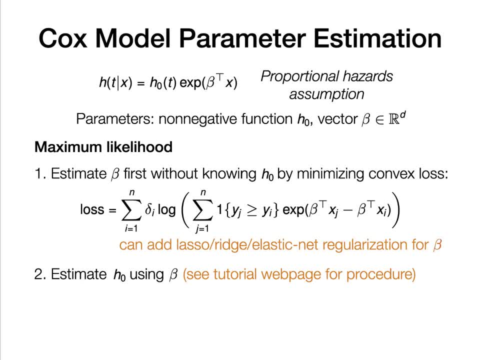 function H sub zero. So I'll just say: look on the tutorial web page for this procedure, It's called the Breslau method. And of course, like I mentioned earlier, after we can back out a hazard function estimate, then we can back out a survival function estimate. OK, 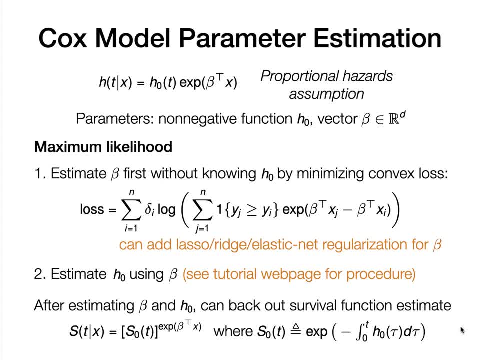 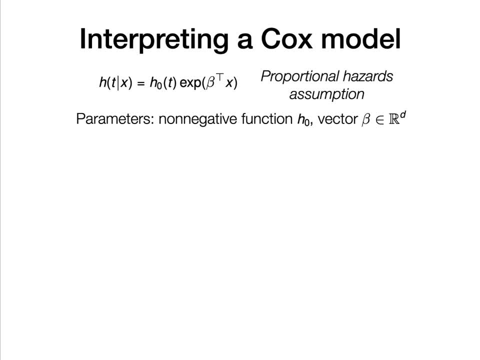 So that's the high level ideas for parameter estimation. The next thing I'll briefly talk about is how to interpret a cost model after you learn the parameters, And I'll just say this is somewhat analogous to linear regression, because, of course, if you're doing linear regression, you're 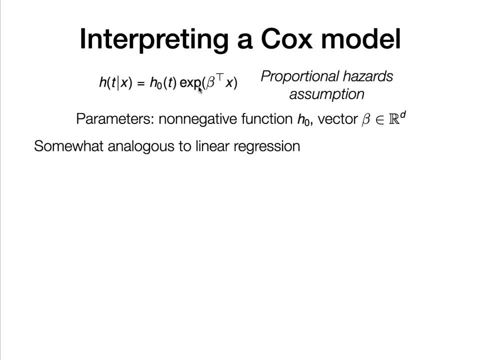 going to be able to do it If you ignore H sub zero and you ignore the exponential. here the beta transpose X part is linear And very commonly what you do is you look at the beta coefficient per feature. OK, where a higher beta coefficient for a particular feature means that that feature 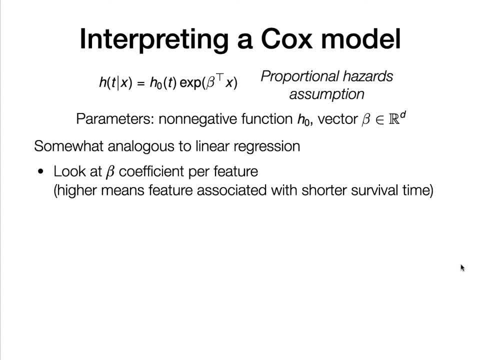 is associated with shorter survival time. OK, because basically the contribution to beta transpose X is going to make the transpose X bigger and again. larger positive values of beta transpose X corresponds to worse survival curves in shorter survival times. OK, so that's what I'll. 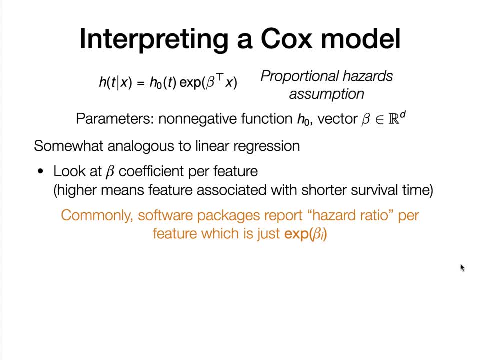 say about that? I would also say that a lot of survival analysis software packages report a hazard ratio per feature and that's just X of beta. I hear beta I is the Cox regression coefficient for the I feature OK. another thing I'll say is: just like in linear regression, 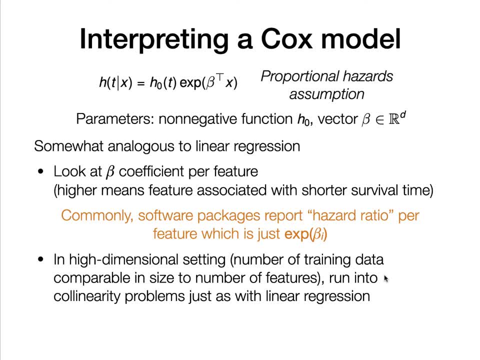 if you're in a high dimensional setting, meaning that the number of training data and is similar in size to the number of features, then you can run into collinearity problems and so forth. So this is the kind of setting where you might want to use. 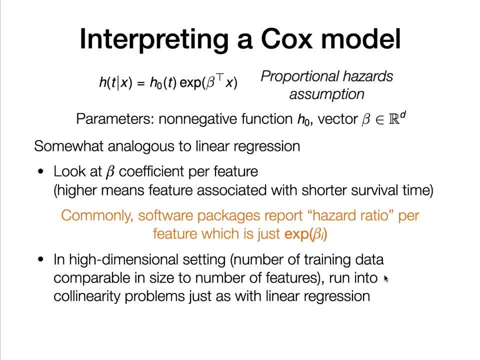 something like ridge regression or lasso or elastic net regularization. OK, so I'll say: unlike standard linear regression, of course we're looking at a hazard function here and I'll say that there is a standard statistical test you can use that's based on what are called Schoenfeld residuals, to check this proportional. 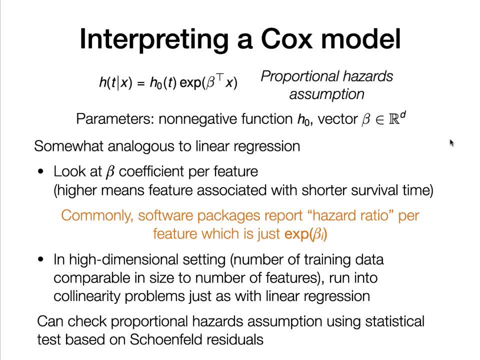 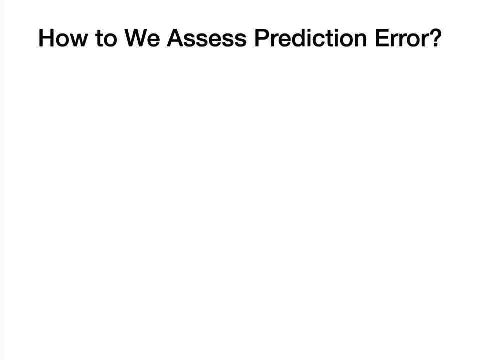 hazards assumption, whether it reasonably holds or not for your data set. So that's what I'll say about interpreting a Cox model. So the next thing I'll talk about is: how do we actually assess prediction error? So here the challenge is that even for our training data we do not actually 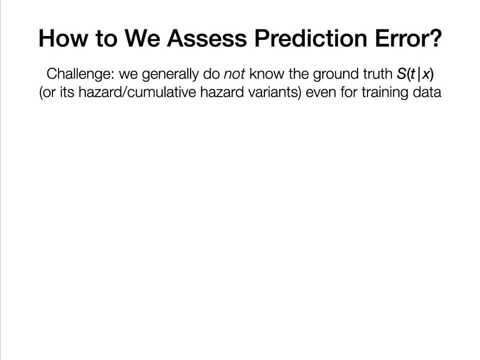 know what the ground truth S of T given X function is, Or the hazard, or cumulative hazard variance, OK, so so what do we do? Well, the key idea is to realize that the Cox model is ranking patients. OK, what do I mean by this? Well, for our training data, the feature vectors X1, all the way to XN. 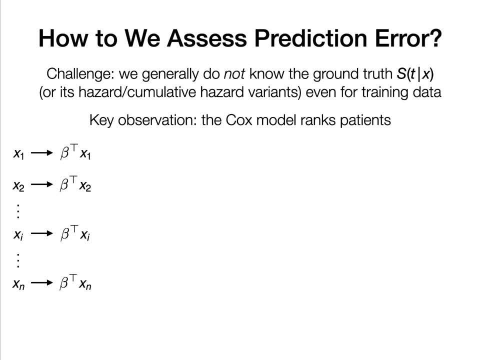 the Cox model after you learn it. basically we're ranking patients by beta transpose of XI: OK. beta transpose of the feature vector, Where higher means shorter survival time or worse outcome, OK. so basically we can use the same idea on validation or test set patients or data points: right Validation or test set data points also. 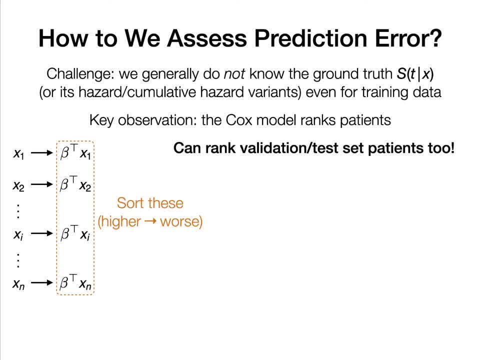 have feature vectors and we can use beta transpose of the feature vector. We can use that to rank, validation or test, set data points And so, in particular, a standard way that researchers we can use to assess prediction error is something called concordance index. 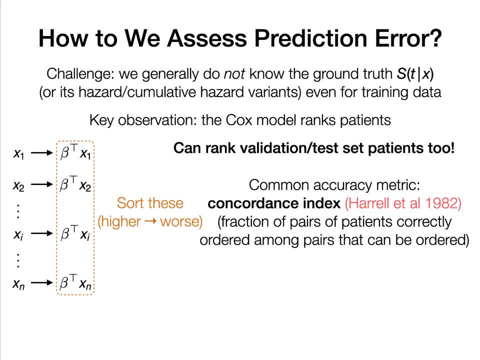 And this is fundamentally a ranking based accuracy metric. OK, and it's going to look at the fraction of pairs of patients correctly ordered among pairs that can be ordered. I'll get to what that means in the next slide, but for now that's what I'll leave it at. So, concordance index, because it was. 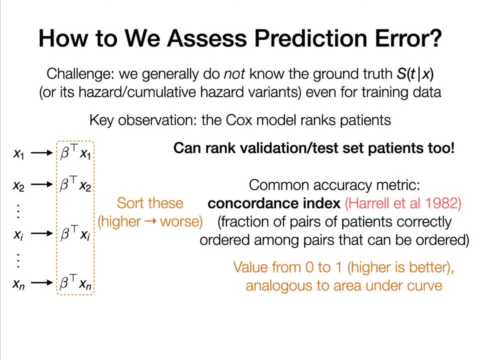 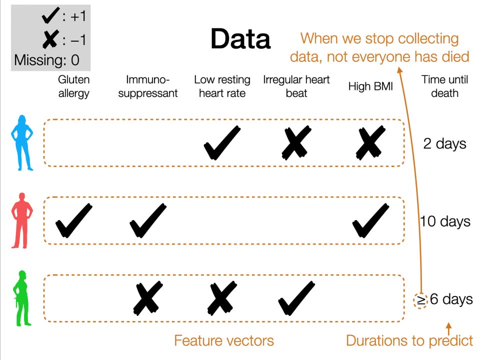 a fraction, it's a value from zero to one where higher is better OK, and in some sense it is like area under the curve for classification. So with that now, I'll say a little bit about what it means among pairs that can be correctly ordered. So let's go back to the example I had. 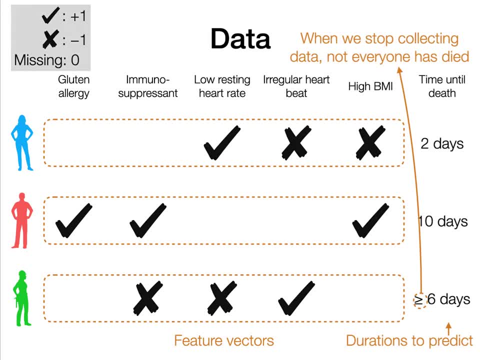 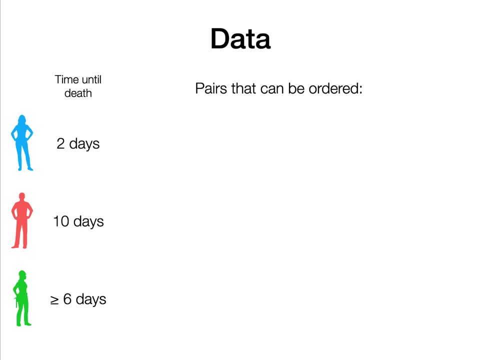 many slides ago for this toy data set here. So for the blue, red and green patients here you can see that I can actually order. For example, I can order blue and red. OK, the blue patient has a time until death. That's well, it's less than that of the red. 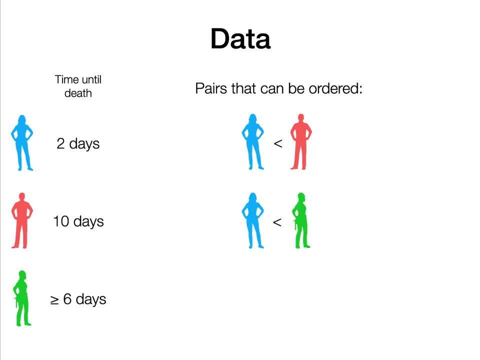 Patient: OK. similarly, I can order blue and green: OK. so, even though the green patient has a sensor time until death, we know that it's at least six, which is considered better than two days. OK. so, however, between the red and green patients, we well, we can't unambiguously order. 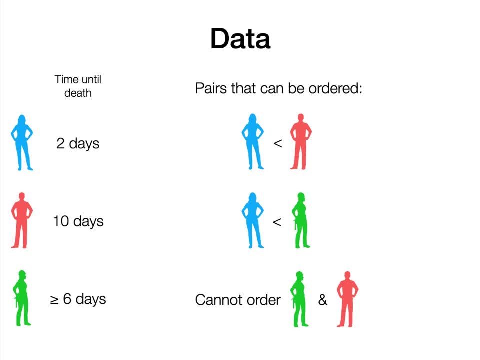 OK, because of the censoring, because of that greater than or equal to sign. So concordance index in this example would look at The fraction of pairs correctly ordered by your prediction method. So if you're using a Cox model, it mean for the beta vector. that's learned. does it correctly rank each of these And, for example, 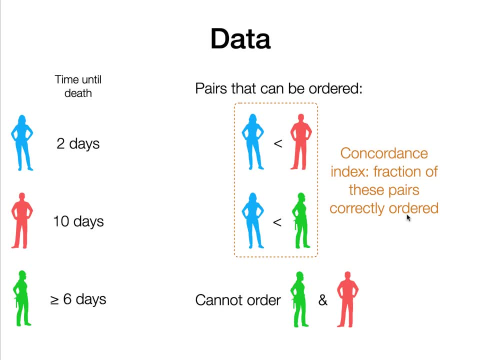 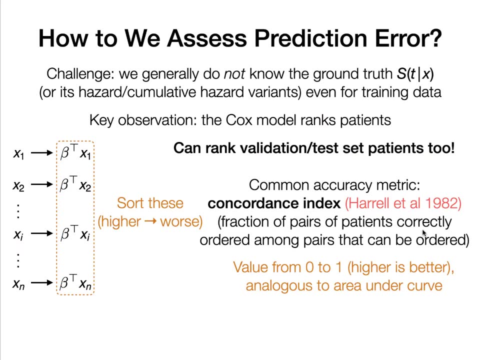 if it ranks only one of these pairs correctly, then the concordance index would be half OK. if it ranks both of them correctly, the concordance index is one. OK, All right. so that's concordance index. I presented it for the Cox model because it's easier to explain. 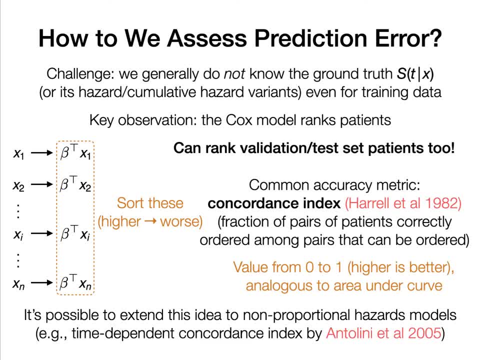 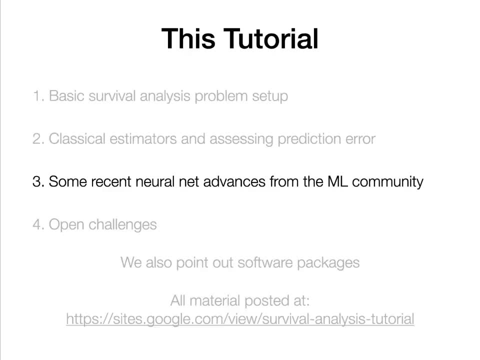 I will say that There is a way to extend this to non-proportional hazards models, And so, as one example of this, there's the time dependent concordance index. OK, that works with other survival models, not just Cox. All right, Now I will talk about some recent known at advances from 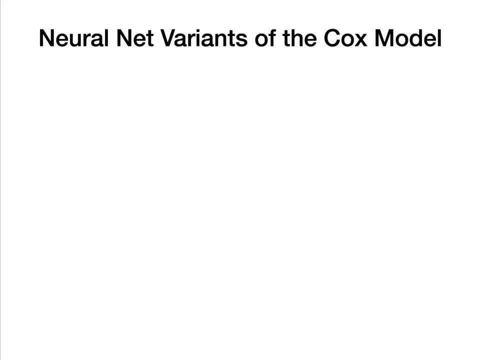 the machine learning community And to begin with I'll talk about some new net variants of the Cox proportional hazards model. As a reminder, the loss function for the Cox model, when we're estimating the Cox regression coefficients, beta, without worrying about the baseline hazard function, H sub zero is given by this equation here And fundamentally, 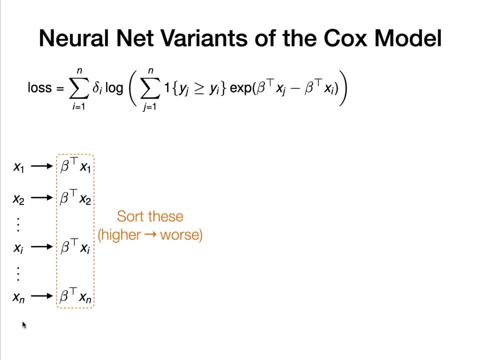 we are learning how to rank the training feature vectors X1 through XN, where we rank them based on the ranking score. beta transpose of X: OK, it's based on inner product, So This turns out to be a ranking loss, And to get a new net variant of this is very simple. 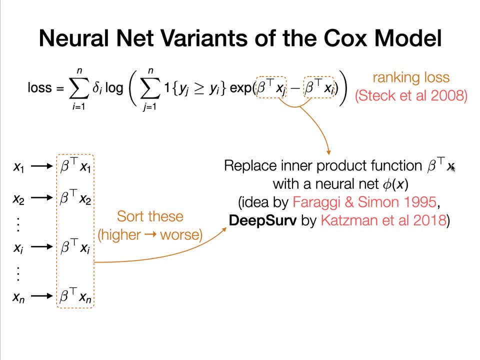 You replace the inner product beta transpose X with a neural net fee of X. OK, And in fact beta transpose X is a special case of a very simple neural net that consists of a single linear layer with no bias and no nonlinear activation. OK. 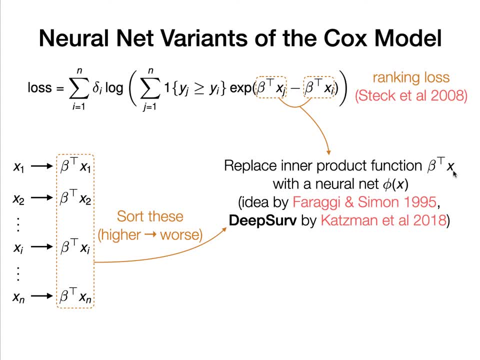 Of course, by replacing beta transpose X with a neural net, you can use something much fancier than just a linear layer. For example, you can use like a multilayer perceptron. or if you have like image structure in your data, you can use a convnet and so forth. 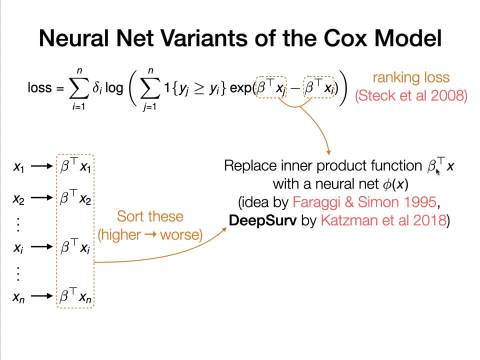 OK, so the basic idea for doing this- replacement of beta transpose X with a neural net- the idea is from the 90s, but there's a recent implementation that's called deep serve. that has become quite popular, And something else you can do, of course, is replace beta transpose X with a neural net. 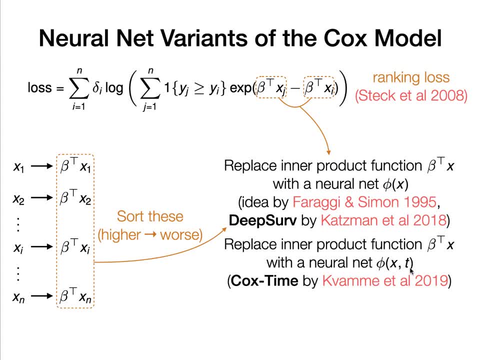 fee of X and the observed time for each data point. Basically, this will give you some sort of time dependence And, as a result, this is referred to as the Cox time model And I'll just say, for deep serve, for Cox time and also for the standard Cox model for this loss function. 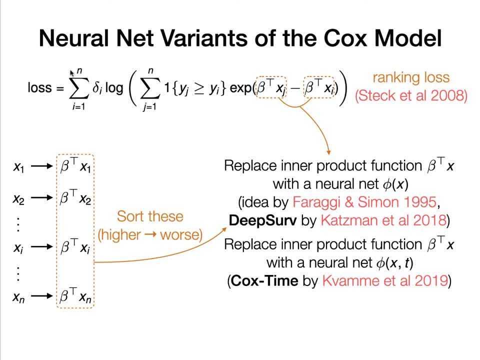 this can be expensive to complete. If the number of training data points and is very, very big in for all three of these models that I just mentioned, you could train them in many batches using many batch gradient descent. to avoid this N squared calculation, However, there's an additional approximation you can do. 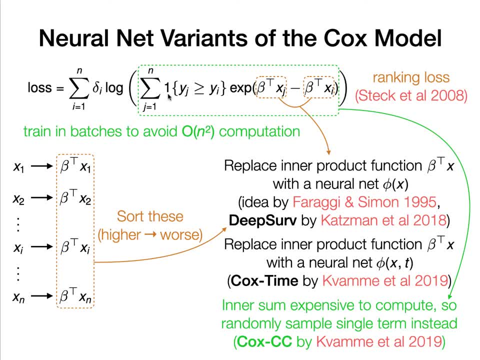 which is to replace this inner summation by randomly just choosing one of the terms in this air summation to evaluate, OK, rather than using the entire sum. And that's what we're going to do, And that results in a model called Cox, CC. OK, the CC stands for case control. 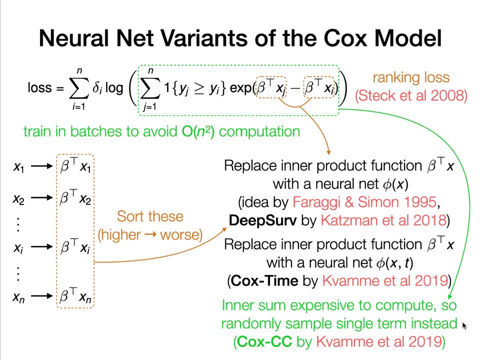 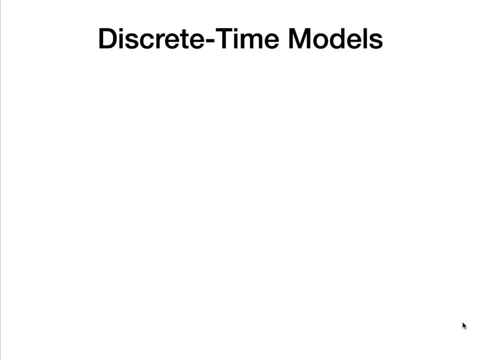 So there you have it: a few different neural net variants of the Cox model. The next kind of model I'll talk about is something referred to as discrete time models, and these are going to estimate a discrete survival curve or some variant of it, such as a. 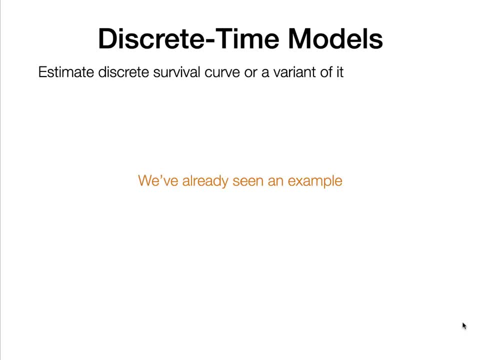 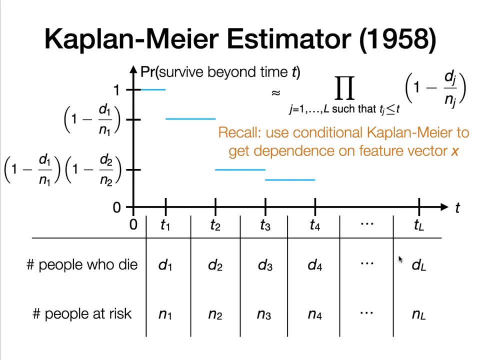 discrete hazard function. So we've already seen an example of this back when I talked about the Kaplan-Meier estimate, And of course it's a conditional variant that depends on the feature vector X And basically what we get out of the conditional Kaplan-Meier estimator and also the Kaplan-Meier 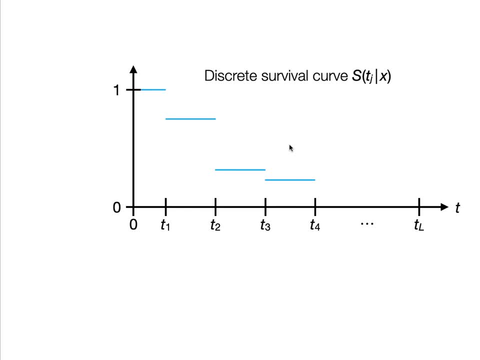 estimator is a discrete estimate of a survival curve. OK, it's discrete because we're keeping track of essentially what's happening at a discrete set of time points. OK, T1,, T2 up to TL, and here also times zero, You can turn a discrete survival curve into a CDF, It turns out. if you do. 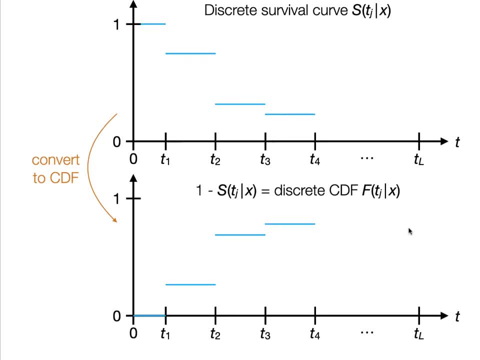 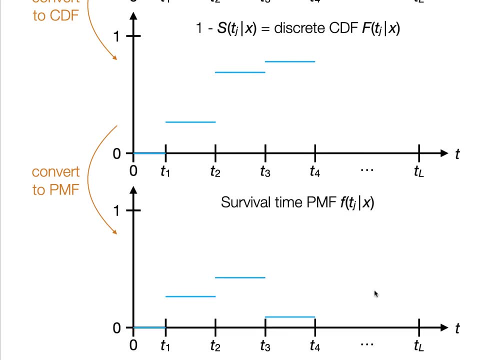 this function, you'll get a CDF. from a discrete CDF, You can back out a probability mass function, referred to as a survival time probability mass function, And from this you can back out a discrete hazard function. OK, using a formula that looks like the continuous time version that I 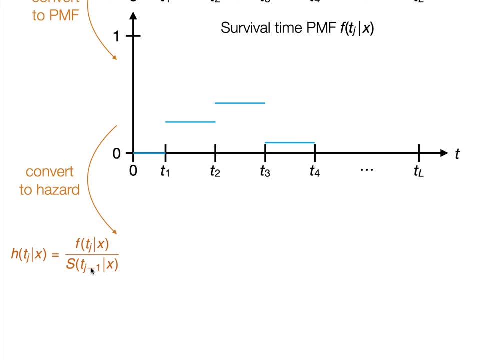 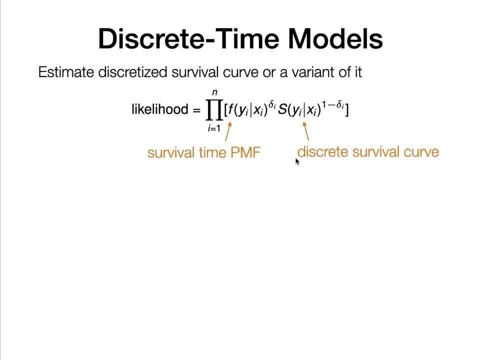 showed many slides ago. that was the instantaneous rate of death at a particular time divided by the probability of surviving beyond time. This is the discrete analog of that continuous time case. In this example, the discrete hazard function looks like this: OK, so by using these discrete versions we can define a likelihood, that's in terms of the. 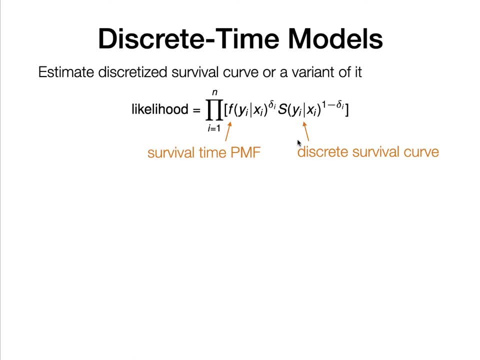 survival time, PMF, in a discrete survival curve And basically you can do maximum likelihood, which of course corresponds to minimizing a negative log likelihood loss, which you can do in many batches. So there are different ways to parametrize f and consequently s and so forth. 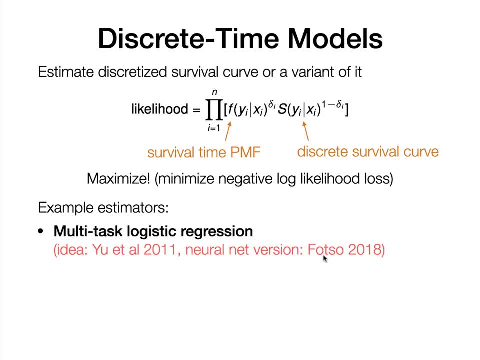 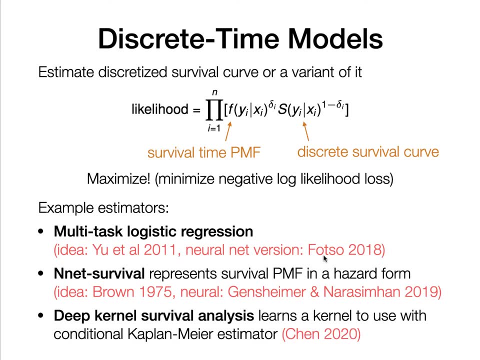 that lead to different models. Some examples of these models would be multitask, logistic regression, the n-net survival model and, lastly, a deep kernel survival analysis. This last model here relates to what we already talked about previously, the conditional Kaplan-Meier estimator I had mentioned. 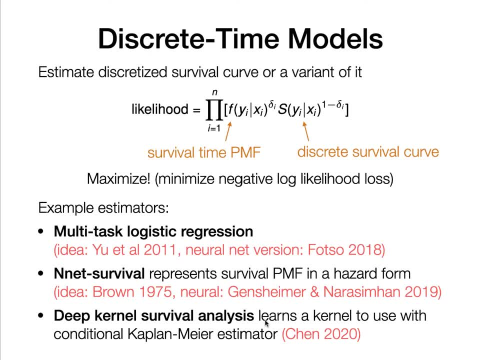 that you can have like a weighted KNN or a kernel KNN, and then you can have a weighted KNN or a kernel variant of it. A kernel variant means you can use a kernel function such as a radial basis function or a box kernel, triangle kernel and whatnot. Deep kernel survival analysis is: 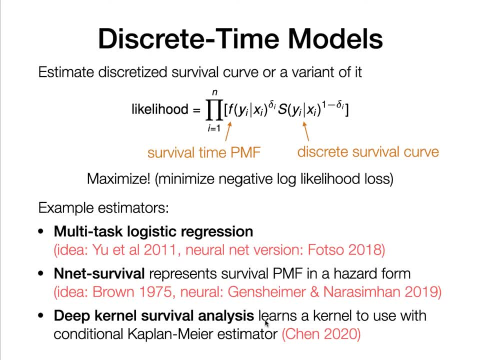 basically just automatically learning a kernel function to use with the conditional Kaplan-Meier estimator, all done in a neural net framework using a discrete hazard function. OK, there is one other discrete time model that I'll mention that I think is very, very good to know, and that's called. 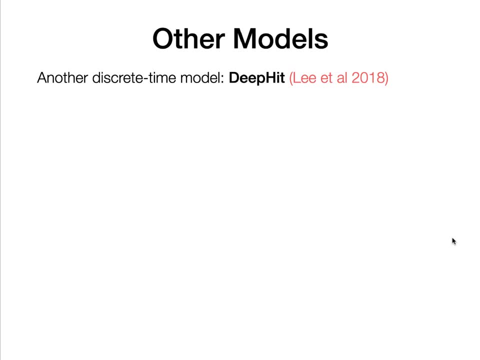 DeepHit. OK, DeepHit is now becoming very popular and it's very accurate in practice, So this models a survival time PMF a certain way, and one of the nice things about DeepHit is that it can also handle a setting referred to as competing events. This is where you have actually 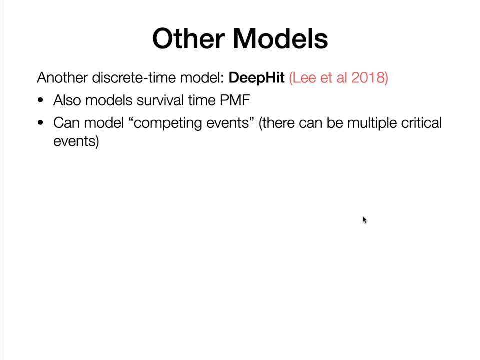 multiple critical events of interest rather than just one. So instead of only looking at, for example, time until death, maybe you're looking at a dataset where you have death as one critical event and also disease relapse OK. so, for example, for a bunch of patients, 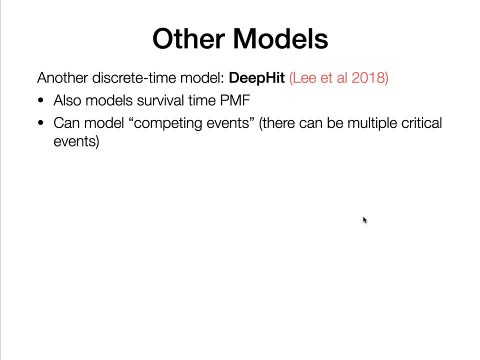 maybe you have time until disease relapse, whereas for some other patients they die before the disease relapses. So that's an example of what's called a competing event. OK, so DeepHit has two loss terms. The first one is like the loss that you saw on the previous slide. 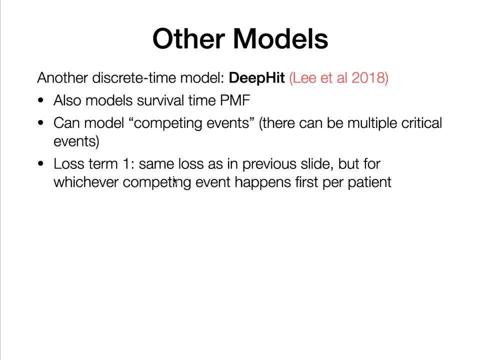 where I was doing that likelihood that you maximize and, of course, is going to be based on a survival time, PMF, because that's what DeepHit amortizes. There's also a second loss term that basically is a ranking loss per competing event. OK, and this ranking loss looks somewhat. 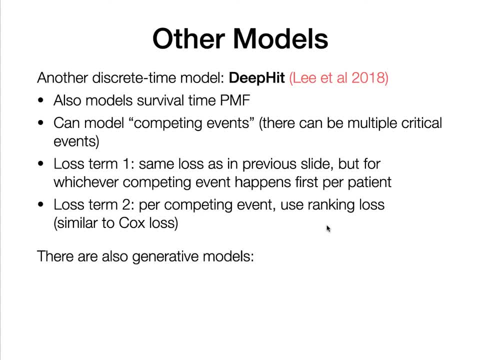 like the Cox loss. I'll also mention, without going into details, that there are generative models. These are basically Bayesian hierarchical models, and examples of this include deep survival analysis, deep survival machines and neural survival supervised testing. OK, I'll see. this last family of models in particular is nice in that it gives you. 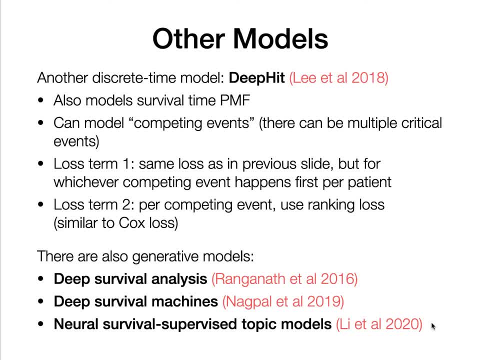 interpretable models- OK, whereas basically these other models I've mentioned that are deep learning based. they can give you very, very accurate prediction results. But typically the models learn can be hard to interpret- OK, whereas neural survival supervised topic models can help you figure out how different features relate and how different topics are. 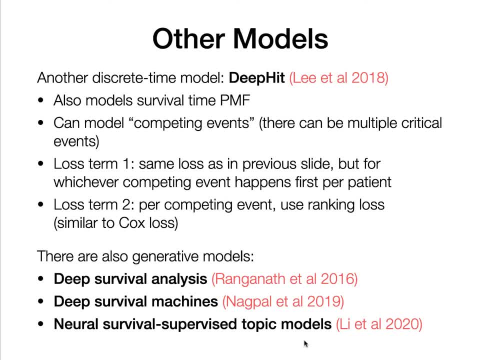 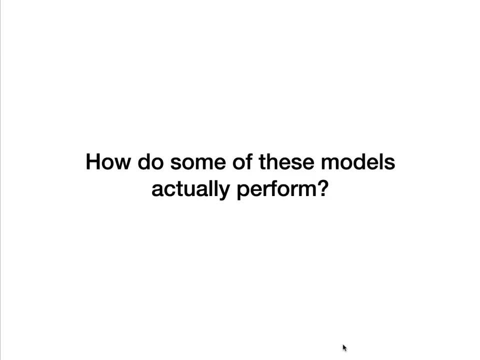 associated With different survival outcomes, and anyways, it can be nicely interpretable, even though it might not achieve the highest accuracy. OK, so that's all I'll say about that. So one question you might have is: how do these models actually perform in practice? 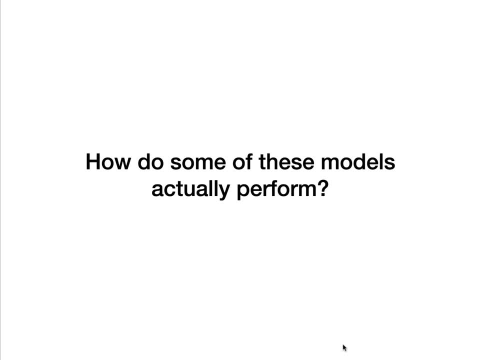 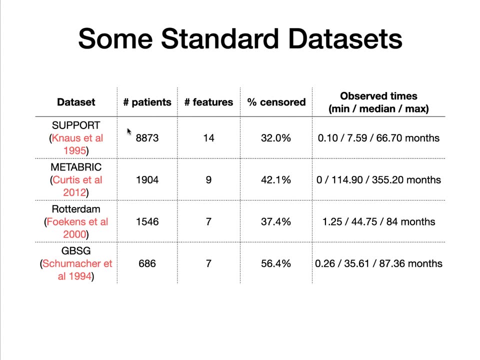 And so I'll show you some experimental results on just a few of these models. I'll show you the results on some standard health care data set. OK, so here we have four data sets commonly used. One is on severely ill hospital patients that have a variety of diseases. 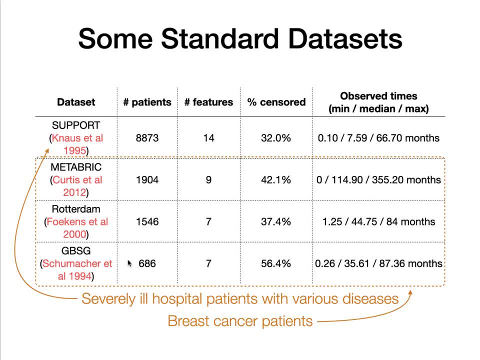 whereas these data sets down here are all on breast cancer patients. For all four data sets, we're looking at predicting time until death. OK, and then here you have, for example, the number of features, censoring rate, some basic statistics on the observed times. 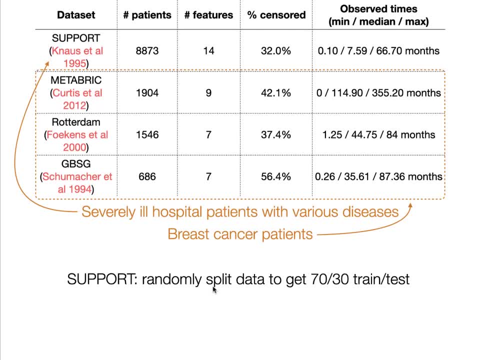 So for the support data set, the experimental results I'll show you. it's going to split the data into a random 70-30 train test split For Metabrick. it'll be the same thing: random 70-30 train test split For Rotterdam and the GBSG data sets. 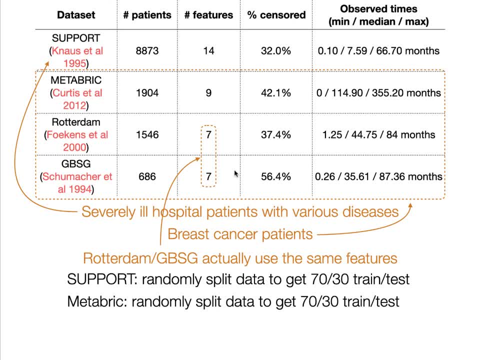 you'll notice a number of features here are the same, because they're actually the same features. One thing you can do- that has been done previously by other authors- is to train on one of these data sets, like train on Rotterdam and test on GBSG. OK, 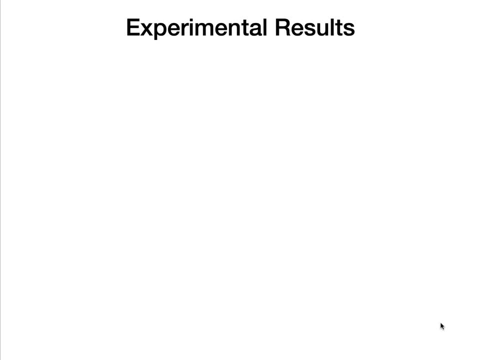 so, in terms of the experimental results, basically, what I'm about to show you is for a bunch of different survival estimators. For each of them I'm going to do five-fold cross-validation to tune hyperparameters. I'm going to select the best one: train on full. 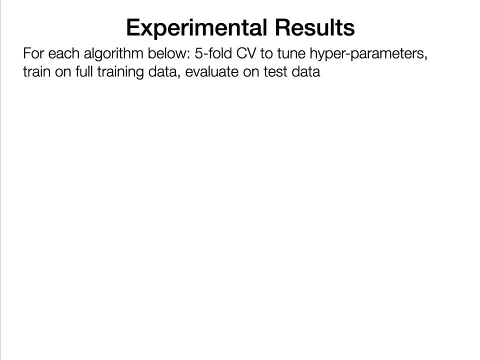 training data set and then evaluate the trained model on the test data. OK, and I'll report test data time-dependent according to indices. So here the different columns corresponds to what? ones for the support data set, ones for the Metabrick and the other ones for the test data. 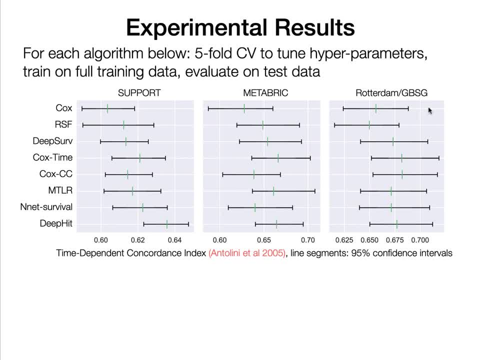 And then the last one is train on Rotterdam test on GBSG. The different rows correspond to different survival estimators. The first two are classical, non-deep learning based estimators: the Cox model and random survival force. The rest of these are all deep learning based survival estimators. OK, 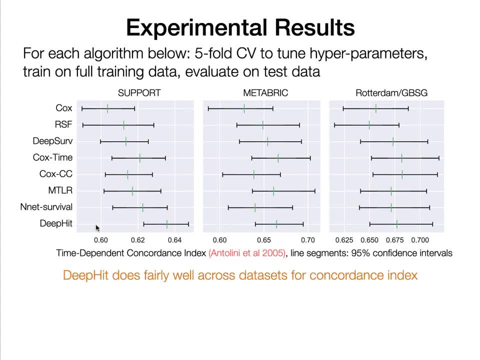 I'm showing this just to give you a sense of the results. Deep hit oftentimes tends to work pretty well across data sets. And then the last one is train on Rotterdam- test on GBSG. And then the last one is train on Rotterdam- test on GBSG. And then the last one is train on Rotterdam- test on GBSG. 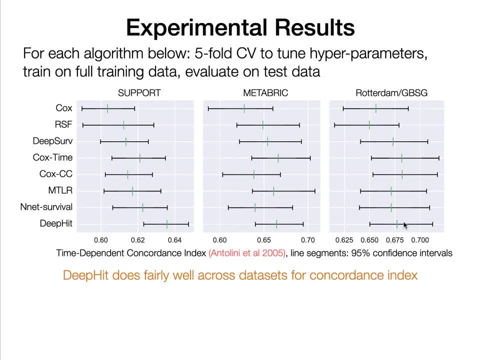 Achieving kind of among the best, if not the best, prediction accuracy, At least for these data sets. none of the methods achieve a concordance index close to one, And I'll just say it's unclear how much better we can do. It could just be for these prediction tasks. they're fairly hard. 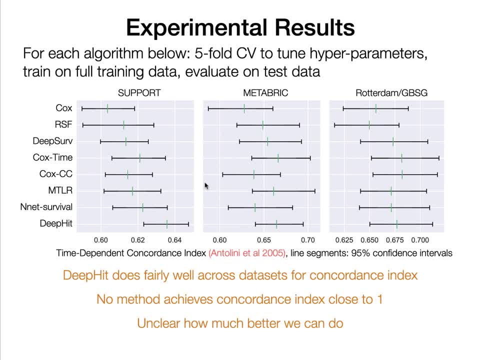 given the features that are present and possibly also given the data set sizes. And something that I'll say again momentarily is that the prediction accuracy for deep learning methods they can be better than classical methods but it could be, you know, not by too much. OK in terms of the 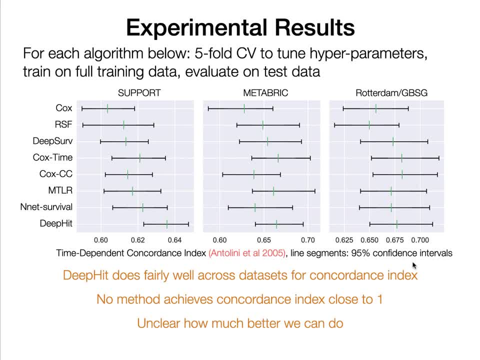 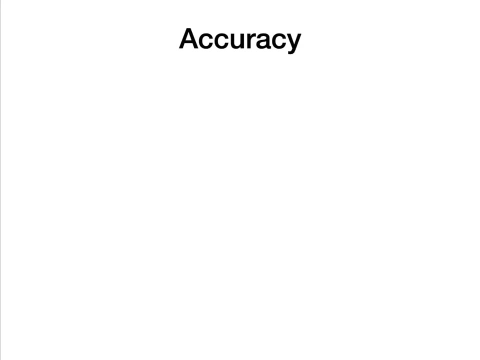 raw absolute differences. OK, so anyways, this hopefully gives you a sense of the prediction accuracy of some deep learning based methods versus classical baselines. Now I'll move on to open challenges, And the first thing I want to get at this is related to the experimental. 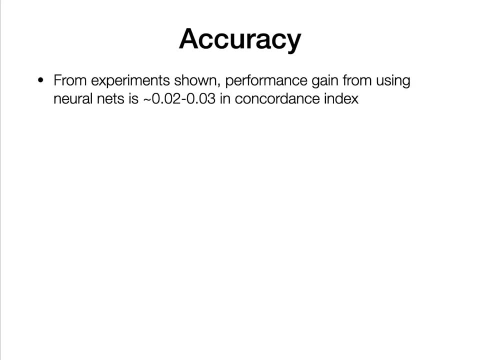 results that you just saw. Basically, oftentimes the performance gain from using deep learning or net-based approaches could be something like 0.02 or 0.03 in concordance index. It's unclear whether this is like a large enough gain for those particular applications of predicting time until. 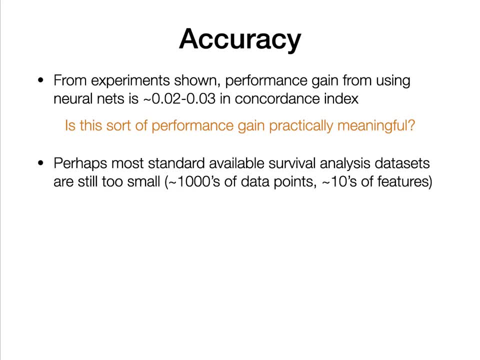 death. One of the issues is that many of the standard survival analysis data sets that are available aren't that big. OK, in terms of, well, the number of data points might be in the thousands. Sometimes, if you're lucky, you might be able to get a lot of data points in the thousands, but 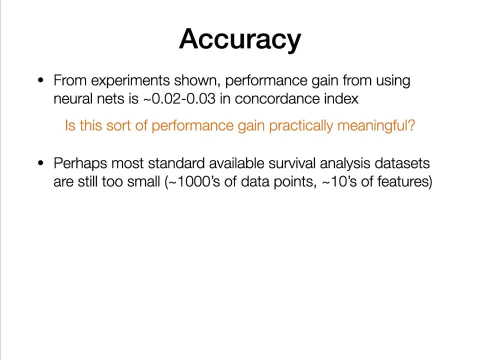 in the tens of thousands or so, the features tend to be like in the tens. Sometimes you might get lucky and be in the hundreds, But really right now, in terms of survival analysis, data sets, the numbers aren't that large And one of the open challenges, I think, is for the communities that 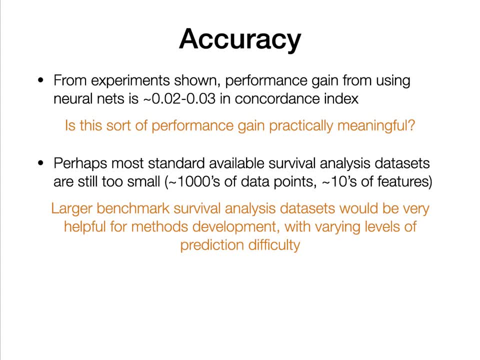 are interested in predicting time to event outcomes to come up with much larger benchmark data sets. I will mention there is one fairly large public benchmark data set I'm aware of. This is data from the music streaming service KKBox, And we're looking at predicting time until users unsubscribe. 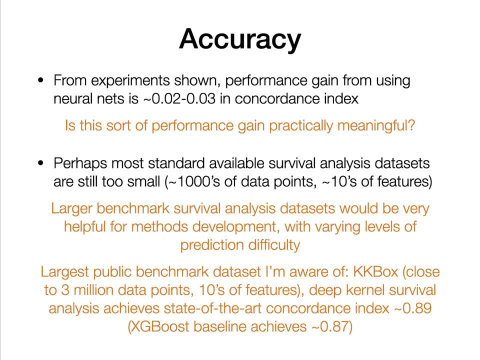 from the streaming service. So this data set has close to three million data points and some tens of features And deep kernel survival analysis can achieve a state-of-the-art concordance index of about 0.89.. And classical non-neonet baseline XGBoost can get a concordance index of about 0.87.. 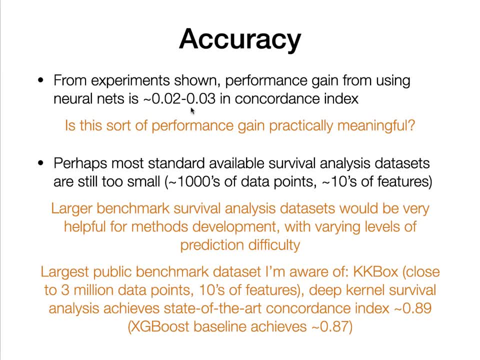 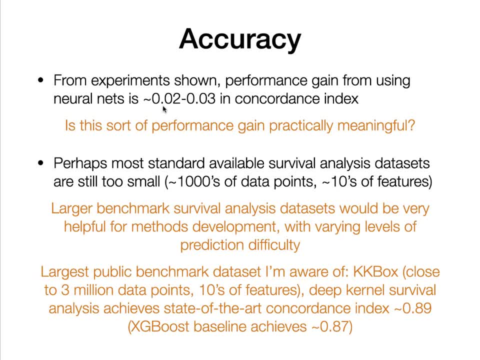 a neonet approach might only be like 0.02 or so, And it's not totally clear whether that's a practically meaningful enough difference to justify using deep learning methods, especially if they can be harder to interpret. OK, at least for this, KKBox data set with concordance indices. 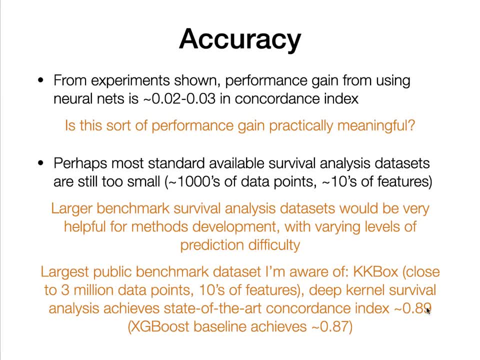 that are fairly high compared to the healthcare examples I showed you. it could be this data set is relatively easy to predict. So I mean this data set is relatively easy to predict. So I mean this data set is relatively easy to predict compared to predicting, you know time. 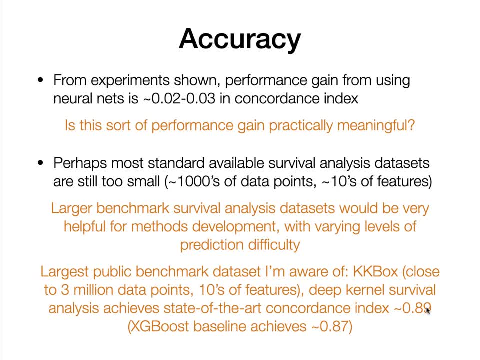 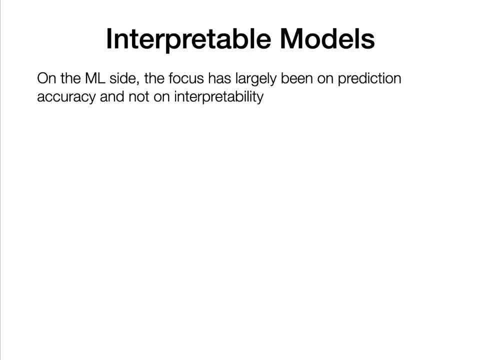 until death, OK, but in any case, that's an illustrative example. Getting back to something I talked about before, a lot of work on the machine learning side has been a focus on prediction accuracy and not so much on interpretability. OK, so if you do want an interpretable model, 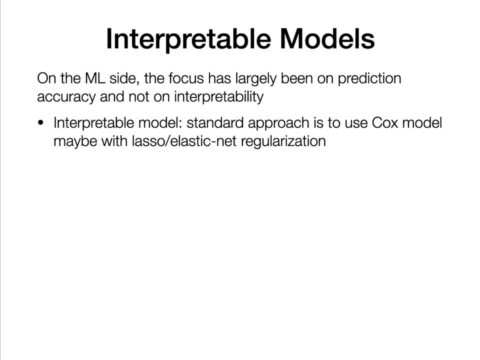 the standard approach is basically to use Cox model, maybe with, let's say, LASSO or elastic net regularization. OK. so if you do want an interpretable model, the standard approach is basically to use Cox model. So again here I'll mention there are other parametric models that people might. 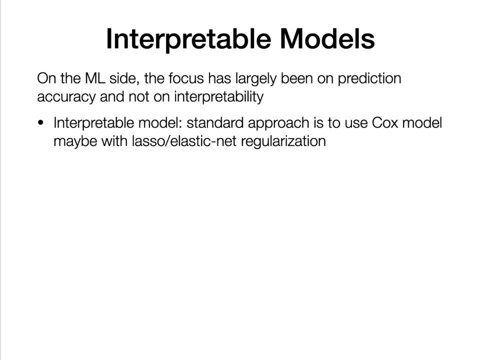 use as well, such as like accelerated failure, time log, normal log, logistic and so forth- models that can also be fairly straightforward to interpret. You can also add LASSO, or elastic net regularization, Deep learning approaches. they can give you higher accuracy than these. 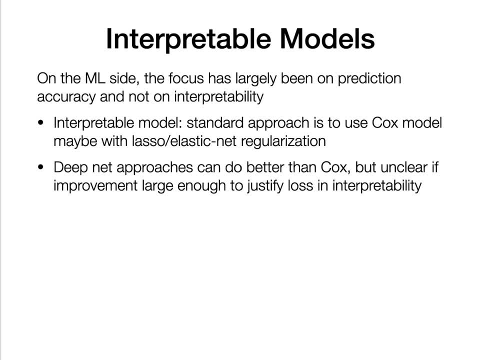 Cox or these other parametric models. But it's unclear if the performance gain, the accuracy improvement, is large enough to justify the loss in the interpretability. okay, So of course it depends on you know whatever application domain you're working in. It depends on a domain. 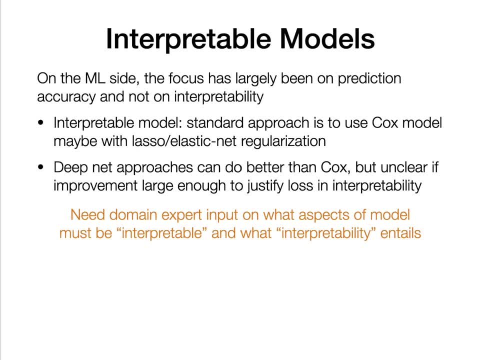 expert to provide input on what parts of the model should be interpretable versus what parts of the model. we don't really care about interpretability and can then use whatever black box models that we want to use to estimate those aspects. okay, This, I guess, is like how the Cox model is. 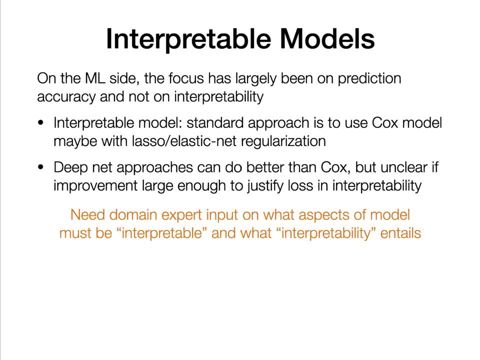 semi-parametric. Some part of it that's parametric is the part we care more about in terms of interpretability. The baseline hazard function is often just something we care less about, so we don't specify a parametric form for it. okay, Of course, it would be nice to have. 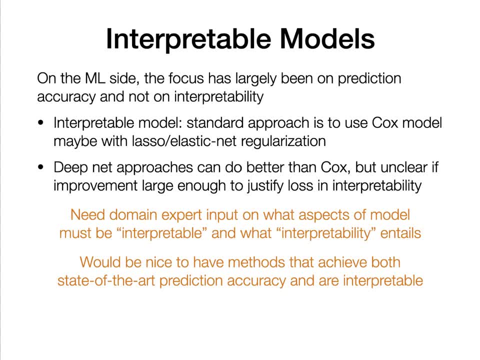 methods that achieve both C of the art prediction accuracy and that are easily interpretable. I think this is an interesting open problem And I'll mention that there has been a lot of work recently in machine learning on explaining black box models. A lot of these ideas, such as 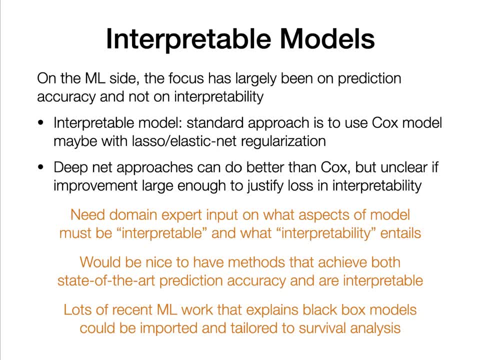 SHAP and so forth could be imported and tailored for survival analysis, but they come with the same pros and cons as they do when analyzing black box models, And some researchers would argue that you should just use an interpretable model to begin with rather than learning an uninterpretable. 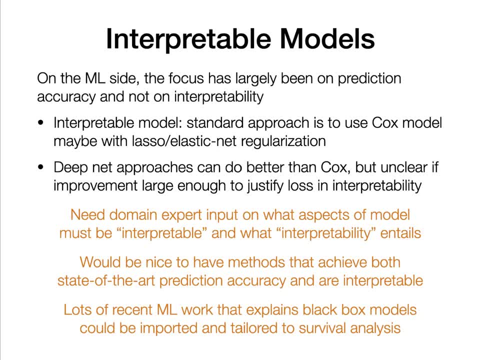 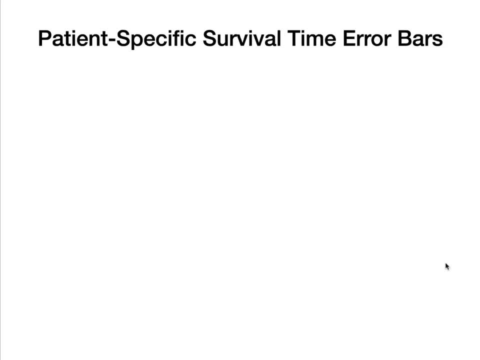 black box that you, after learning the model, you use one of the other models. Okay, so something I'll mention that I think is interesting for the community to think about more is survival time error bars. okay, So it turns out that it's now possible to construct: 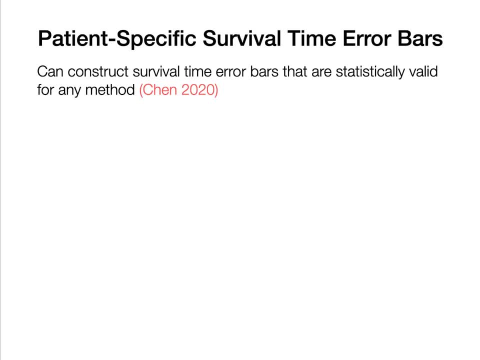 survival time error bars that actually are statistically valid, okay, And an example of this would be something like: oh, we predict, let's say Alice, to have, with probability 90% survival time, 30 plus or minus 20 years. okay, So here this 90% is referred to as a coverage. 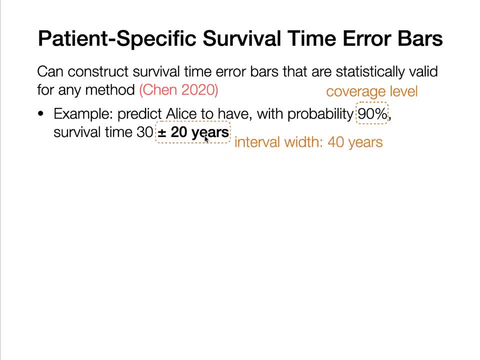 level In this: plus or minus 20, this is like an interval width. Here the width is 40 years. okay, Basically, these are like confidence intervals. Well, confidence intervals are for the model parameters, whereas here we're looking at prediction intervals. okay, So basically, 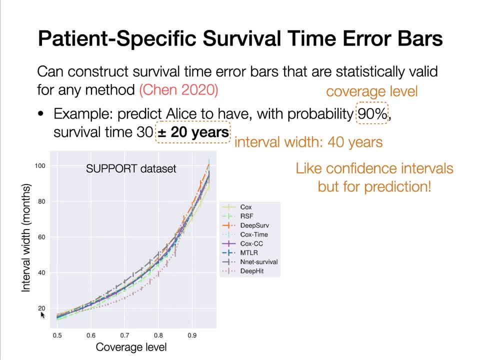 what you can do is you can plot prediction interval width as a function of coverage level. okay, You can compute this for any survival estimator you want, and this is an interesting way to look at. depending on what interval width you want or what coverage level you want, you can see. 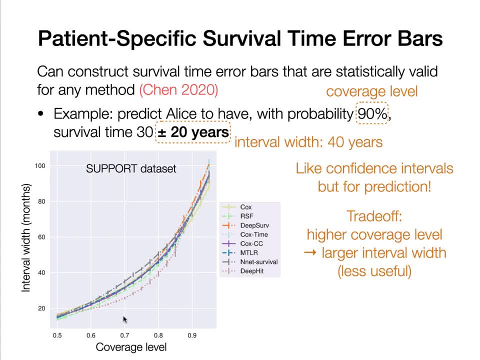 what kind of model achieves, you know, the lowest interval width. for example, Let's say you're like: oh, I want a coverage level of 70% and I want the lowest interval width possible. What achieves that? In this example, it'll turn out to be: 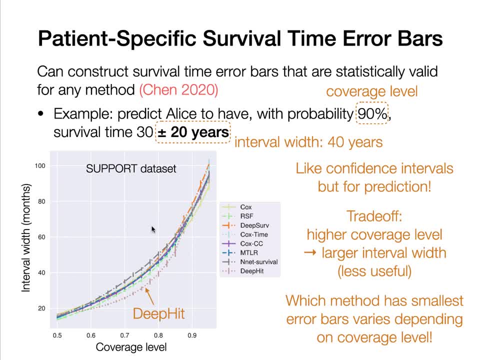 uh, deep hit okay, Whereas if you want a high coverage level and as low of an interval width as possible, it will be a coxmo okay. So I'll just say here there's a tradeoff that's similar to confidence intervals, as you might know. if you have like a 90% confidence, 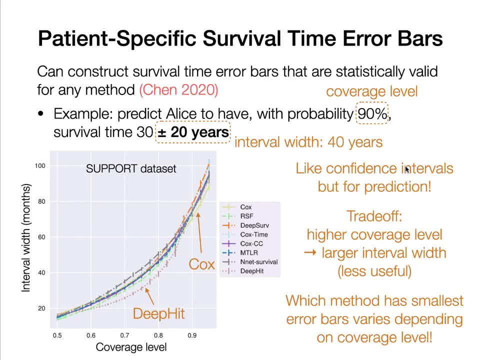 interval versus a 95% confidence interval. as you make the coverage level larger, your interval width become wider, which means that the interval you have is not as useful when it's wider. So there's a trade-off between um interval width and coverage level. So 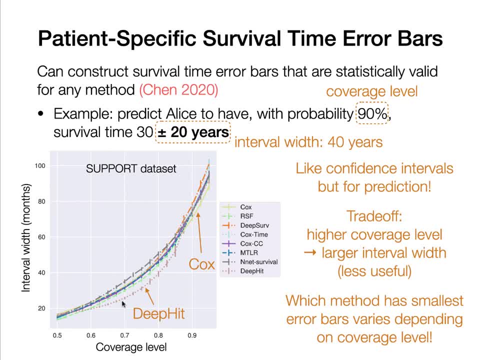 the interface that you want to map. we can see that that was critically modified. yes, that was significantly modified. And now you will want another tradeoff. You could start på für 단式Оn Rmışa coverage level. a plot like this can help you decide on what model to use. okay, all right, cool. 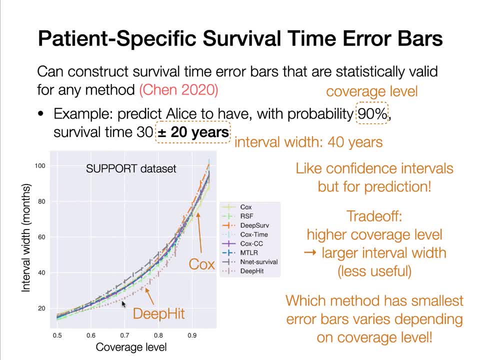 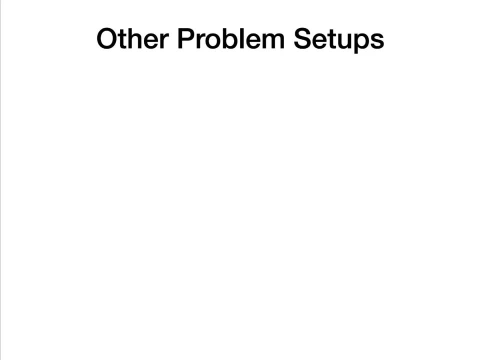 so that's what i'll say about this, and this kind of idea is, uh, not yet all that popular, but i think it is a valuable way to view a bunch of these prediction problems in survival analysis. so some other things i'll talk about is that there are some other problem setups that we didn't talk. 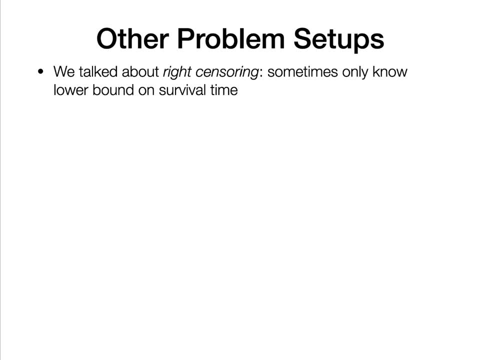 about: uh, so we specifically focus on talking about right censoring. this is when you have that greater than or equal to sign, so a lower bound on survival time. but it's also possible to have left censoring where you have an upper bound on a time, so this could be like time when a child 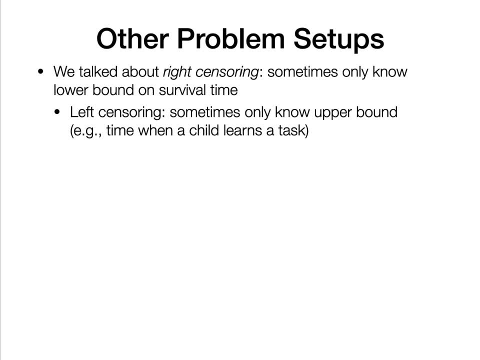 learns a task, you finally observe: oh, this child can do something. basically, they learned it before you know for sure. they learned it the exact time when they learned the task can be censored. so uh, i'll just say it's possible to modify right censoring methods to work with left censoring. 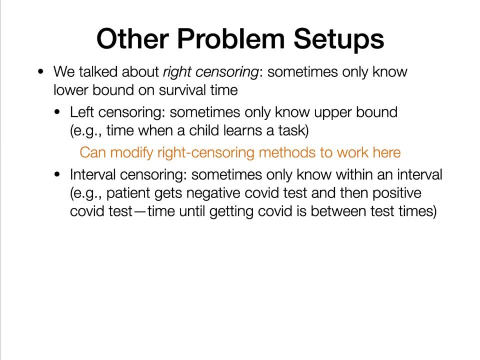 also commonly you might have something called interval censoring. okay, this is where you know that the critical event happened within an interval, but you don't know exactly when in that interval. okay. so, for example, a patient gets a negative covid test and then gets a positive covid test, then you can say, well, time until getting covid is, it's within an interval. okay. 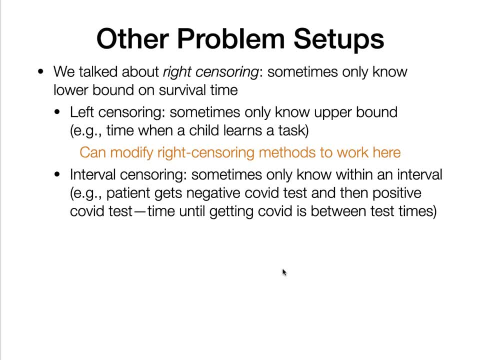 but we don't know the exact time. so, uh, yeah, i'll just say there are some methods for dealing with this. um, some other things that i didn't really talk about is that feature vectors can have missing values and uh. so there is an issue of how do you deal with imputation. i guess much earlier. 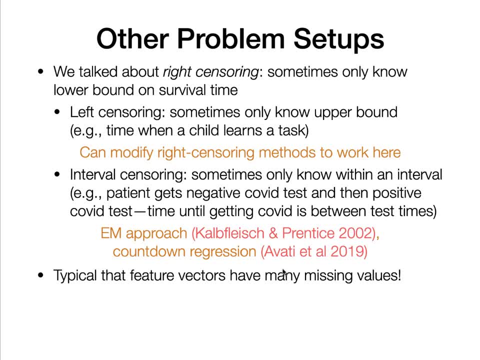 i had an example where i just filled in all the missing values of zero. that might not be what you want to do in a lot of practical scenarios. um, something else is: oftentimes you might be doing a time to event prediction task where time dynamics matter. okay, 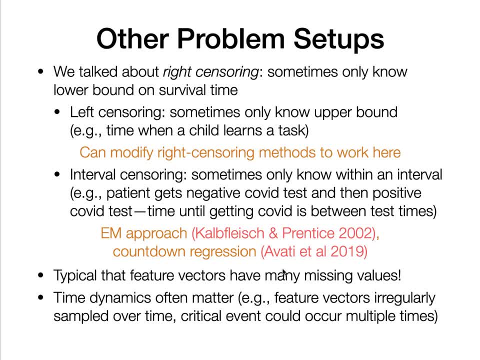 maybe you have feature vectors that are actually sampled over time and, uh, maybe they're irregularly sampled over time and you want to, at different time points, predict time until a critical event happens. okay, so i'll just say there are a bunch of researchers now that are working on these kinds. 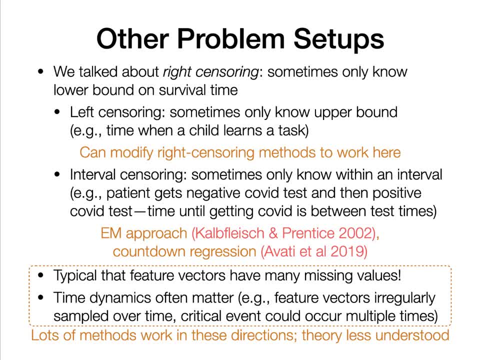 of methods. the theory here is less well understood and, as you can imagine, it's much more complicated. that's all i will say about other problem setups. now i will say that i'm not sure if i'm going to be able to do this all on my own, but i'll just say 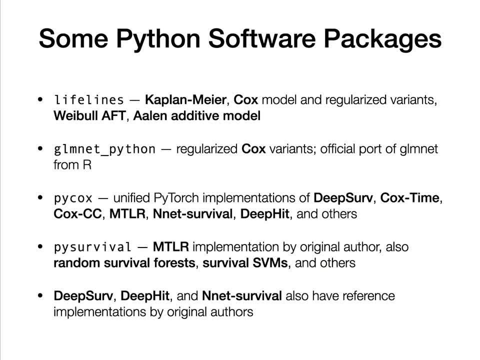 give a very inexhaustive list of software packages available, starting with some packages in python. here we, for example, have lifelines, which implements a bunch of classical models, including a few that we talked about, such as the kaplan meyer estimator, the standard cox model and also. 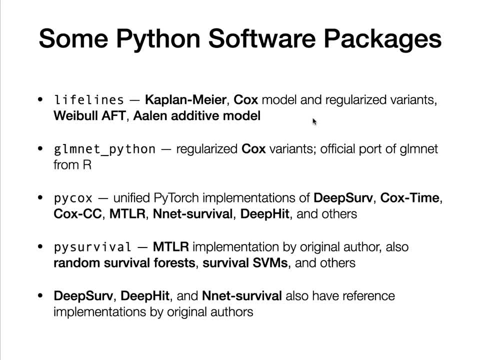 regularized variants of the standard cox model. there's separately a fairly robust implementation of regularized cox models that's referred to as glmnet python. this is the official port of a very popular package in r called glmnet. that includes regularized cox variants. okay. 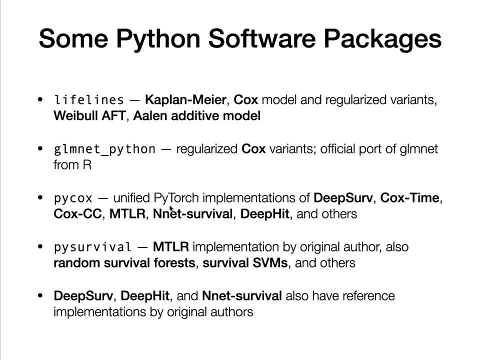 next up, we have pycox, which provides a unified framework, including pytorch implementations, for a whole bunch of different neonet based survival estimators. okay, this is very nice because it's a unified interface for a bunch of these models and also a bunch of different data sets. in fact, the experimental results i showed you earlier were implemented. 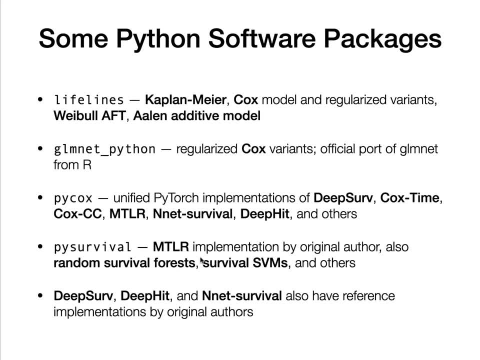 largely in pycox. next up we have pi survival. this includes a reference multi-task logistic regression implementation by the original author, as well as python implementations of random survival for us, which i mentioned. okay, as well as some other uh classical models. um, i'll mention that some of the neural net based methods, such as deepserv, deep hit and net survival, 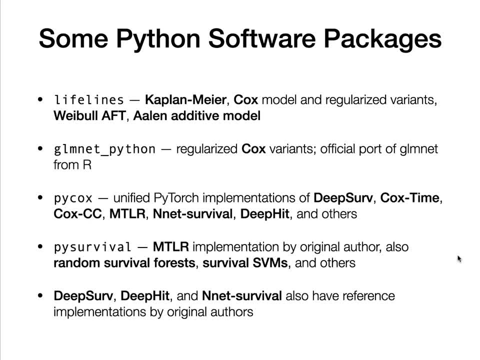 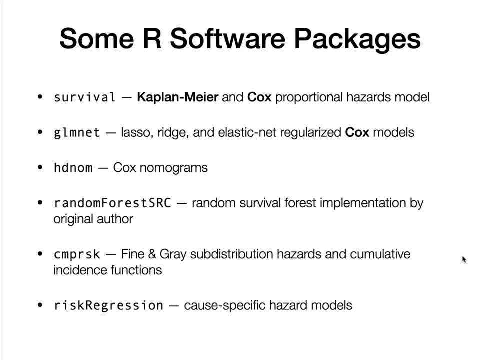 also have reference implementations by the original authors. okay, moving on to some r software packages. for the most part the r software packages are for classical models rather than neural net based models. okay, so you have your usual implementations for kaplan, meyer and standard cox models. as i 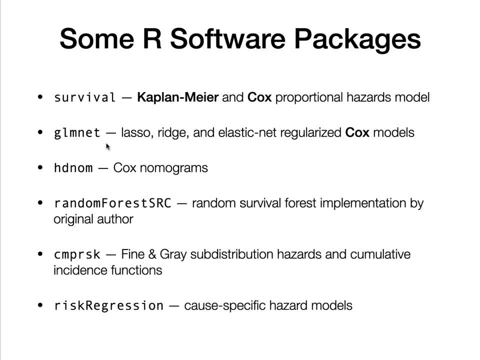 mentioned in the previous slide, we have a lot of models that are more like native models, which are. there's something called GLMNet that includes very robust implementations of regularized Cox models. There's also something cool called HDNOT. This is for making nomograms. This is a simple visualization you can create to help.